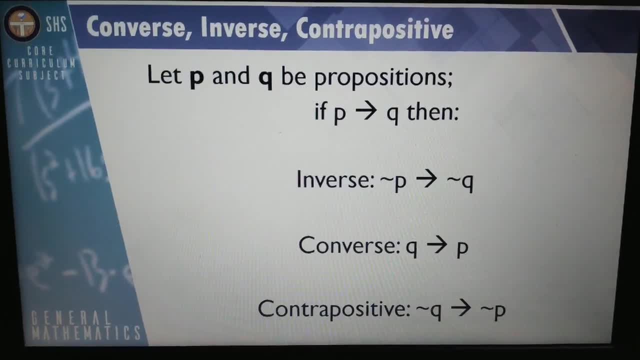 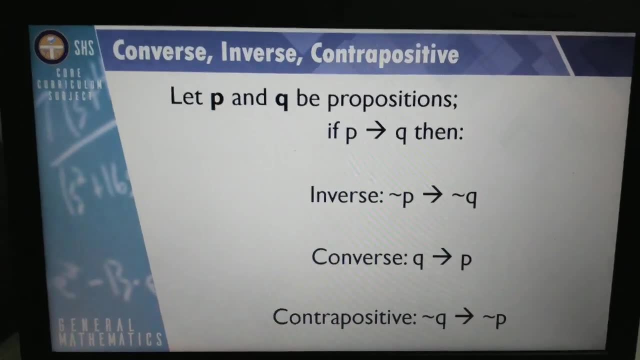 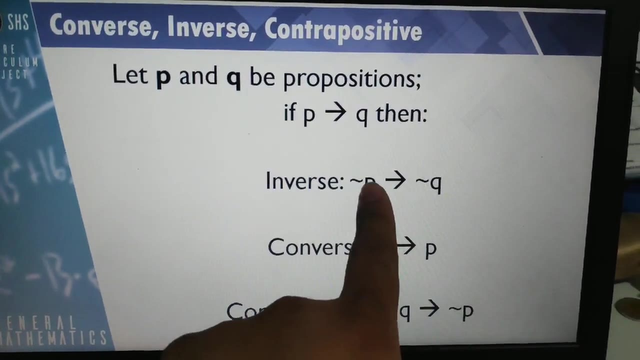 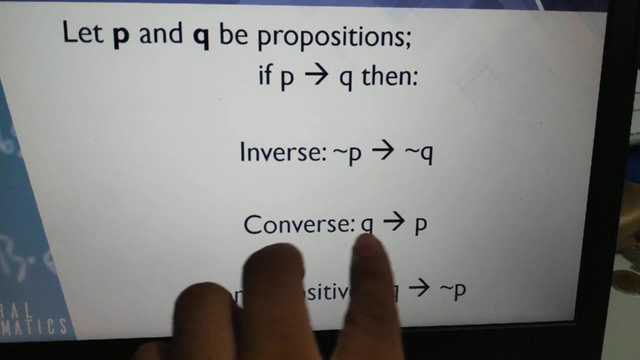 but first let's start with the concept of converse, inverse and contrapositive. let's say you have two propositions, P and Q. then if we have the conditional statement P to Q, then the inverse would be negating statement P and negating statement P- Q. now for converse, you are just going to flip the two statements together for 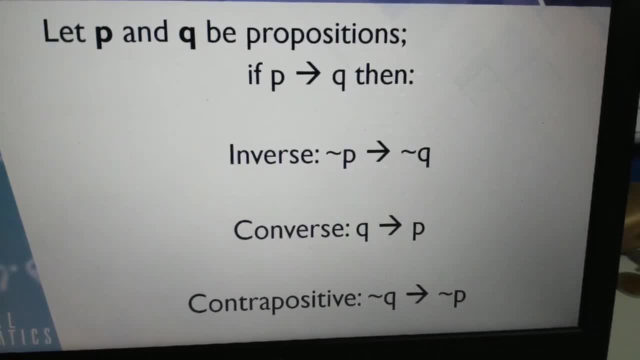 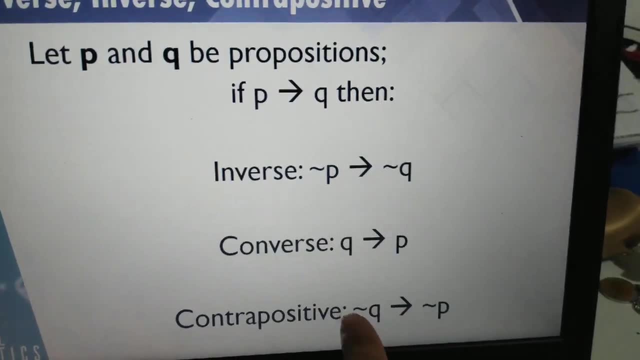 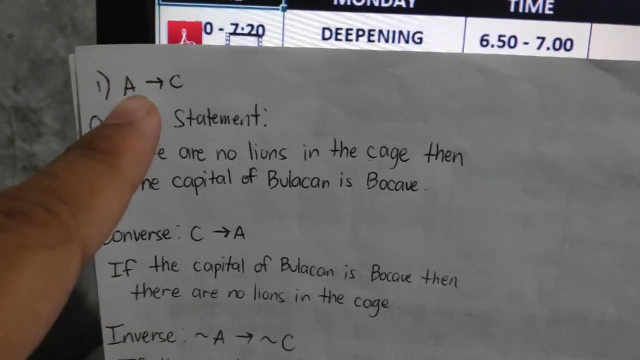 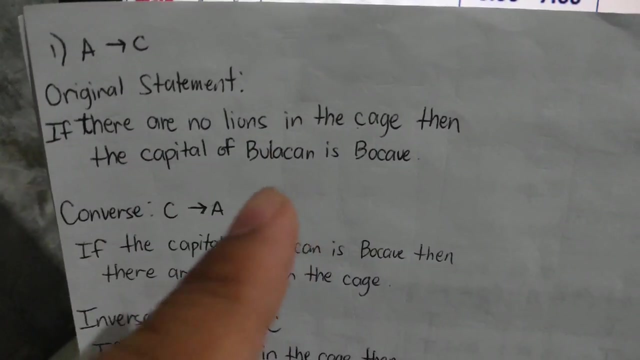 it to get the converse and for the contrapositive from the original conditional statement, you will flip the two statements and then you will negate them. so here the example we have: statement A implies statement C, so for the original statement it will be: if there are no lions in the cage, then the capital of Bulacan is Bukawe. now for. 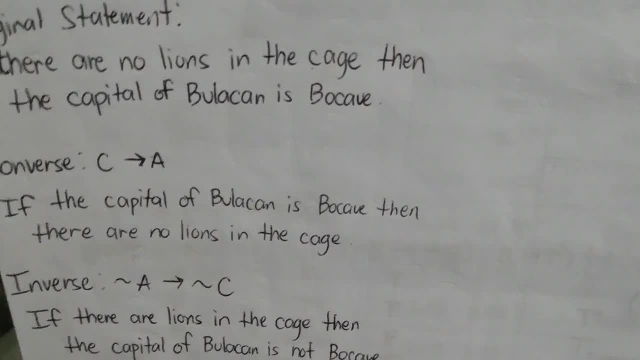 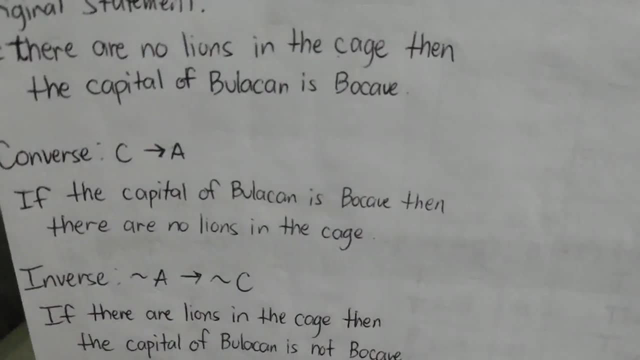 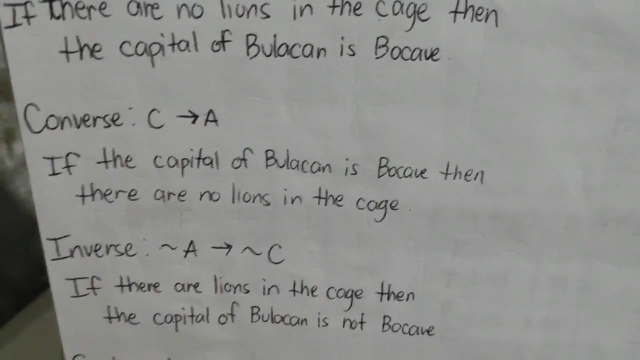 the converse. as stated earlier, you will just get or switch the position of A and C, so the converse of A implies C becomes now C implies A, so the converse will be: if the capital of Bulacan is Bukawe, then there are no lions in the cage. 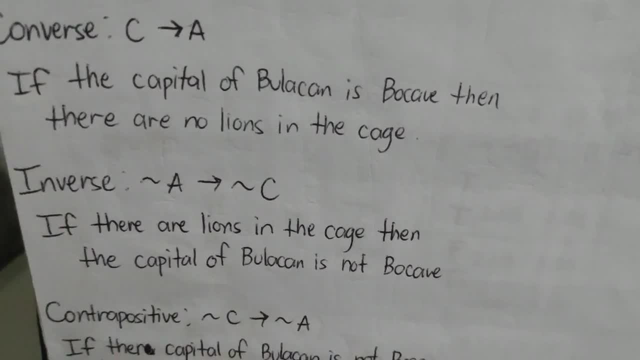 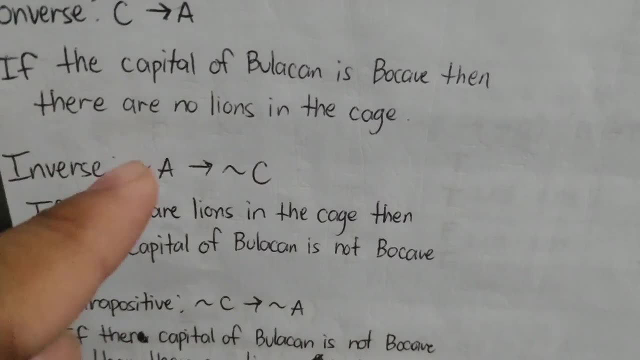 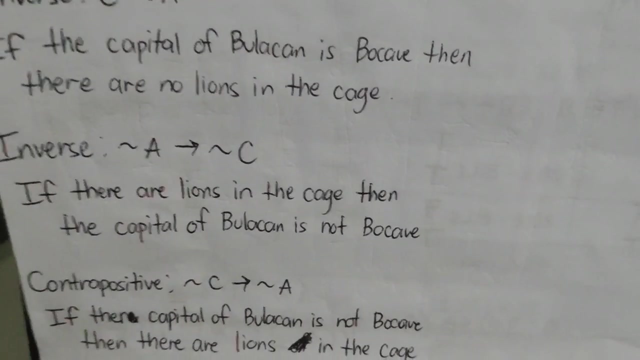 and now for the inverse. it will be just negating the original statement. so you will negate A and negate C, so the resulting will be: the negation of A implies the negation of C, so the statement will become: if there are lions in the cage, then the capital of Bulacan is not Bukawe. now for. 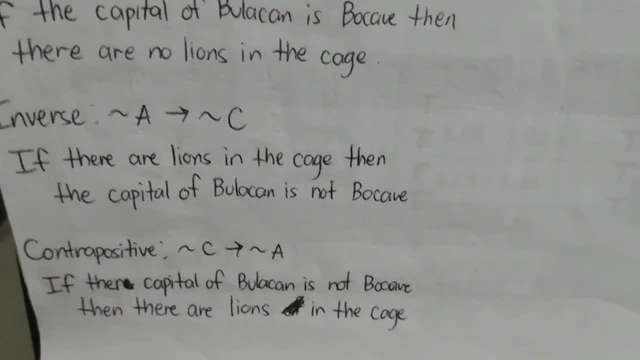 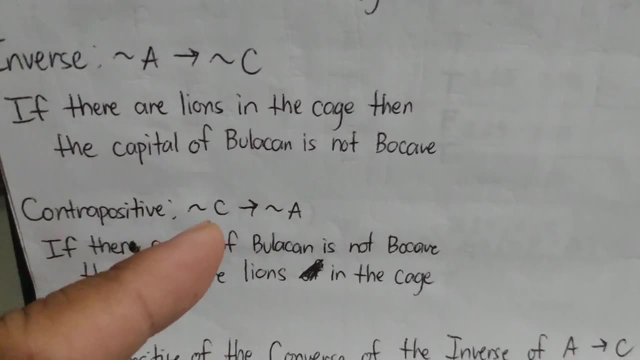 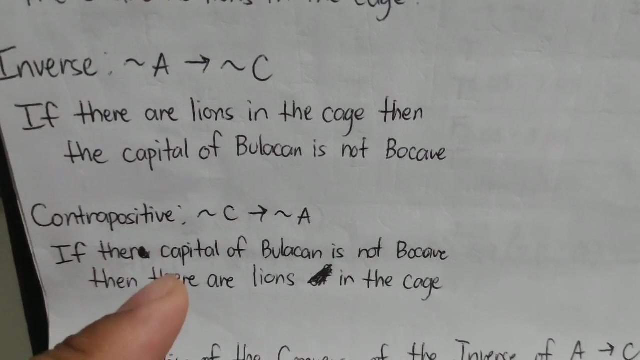 contrapositive, you will switch the original statement A implies C to become C and Bukawe will become C implies A- and then negate them, so it will become the negation of C implies the negation of A. so the statement will become: if the capital of 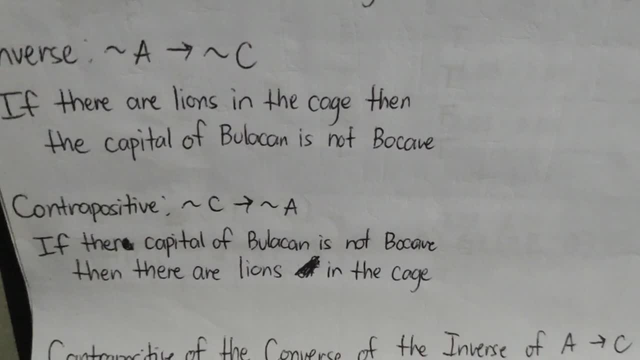 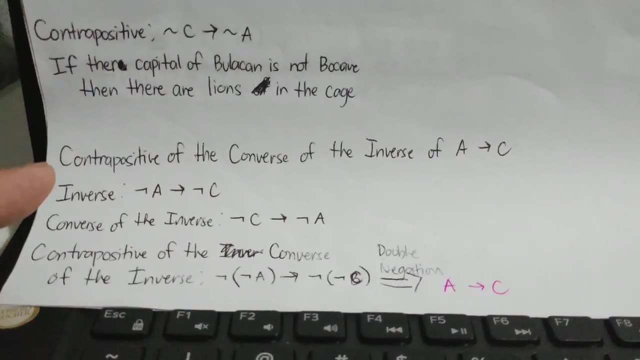 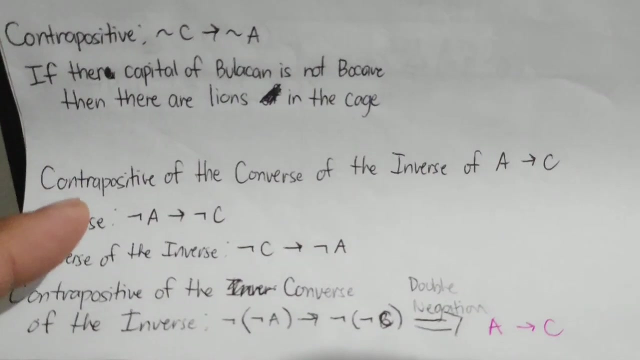 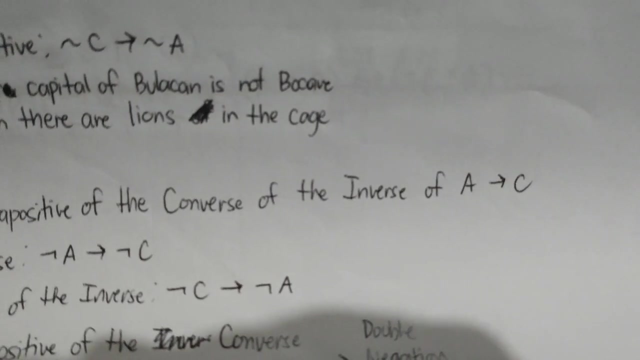 Bulacan is not Bukawe, then there are lions in the cage. so if we now have the combination for the different forms, forms of the conditional statement, so what is the contraprositive of the converse, of the inverse of A implies C. so how would you go about it? 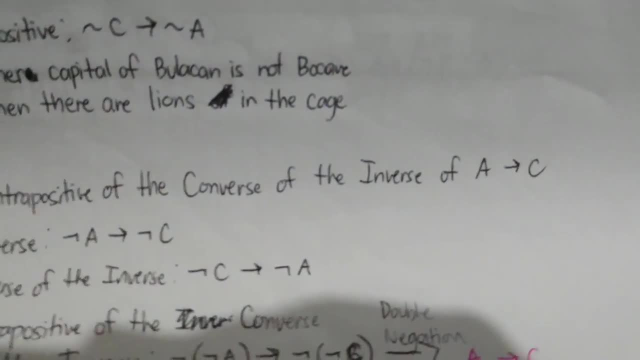 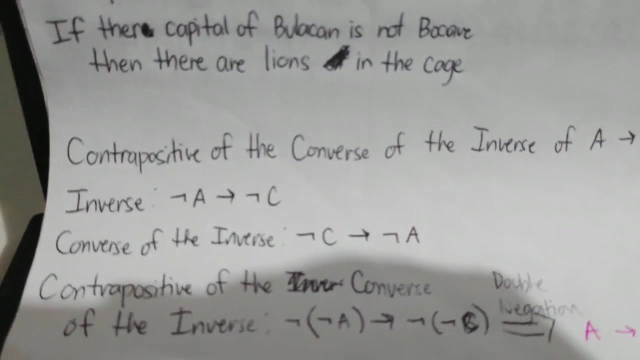 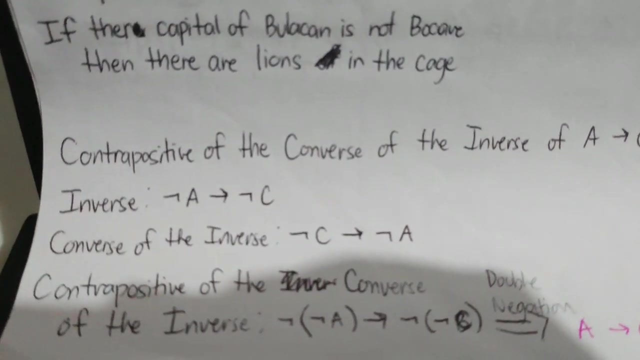 so first get the inverse of A implies C. so the inverse of A luggage A implies C. simply negating the two propositions. so you will have the negation of A implies the negation of C. now for the converse of the inverse, you will just switch the. 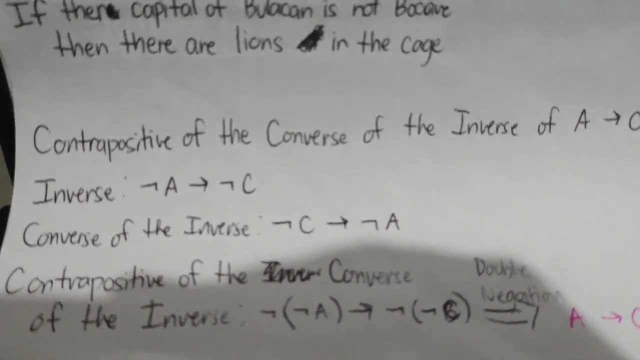 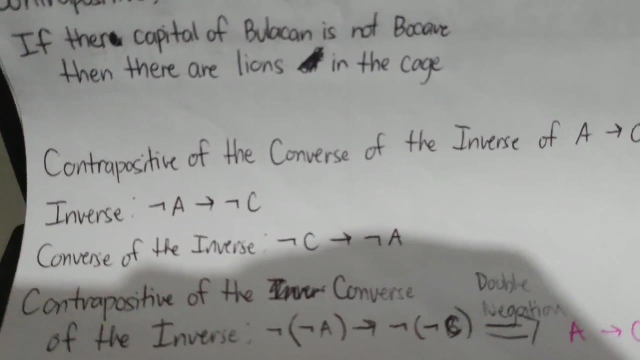 position of the negation of A and negation of C of C, So the converse becomes: negation of C implies the negation of A And the last will be the contrapositive of the converse of the inverse. So from negation of C implies: 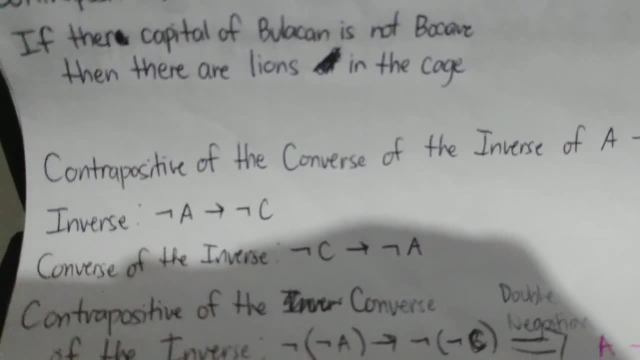 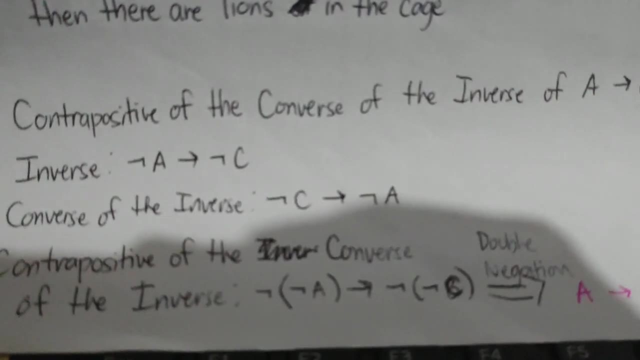 negation of A, you will switch the two, So it will become: the negation of A implies the negation of C. But since you are getting the contrapositive after switching them, you will negate them. So you have the negation of. the negation of A implies the negation of the. 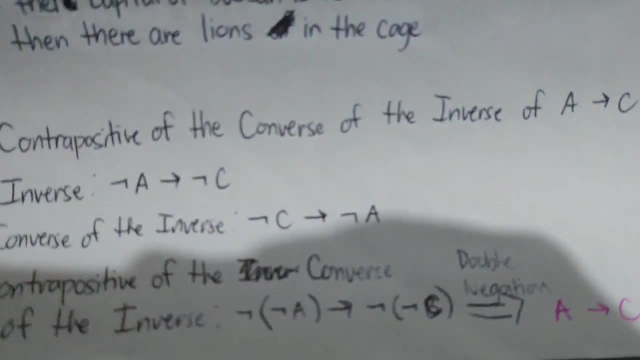 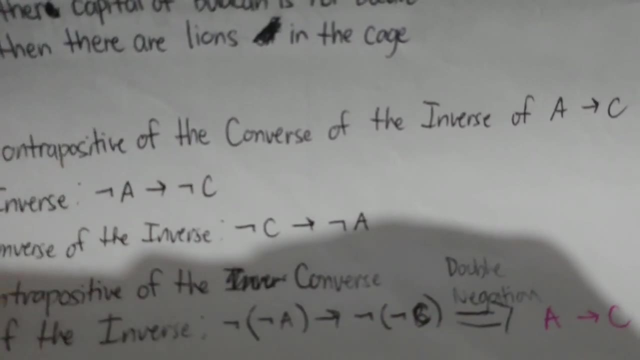 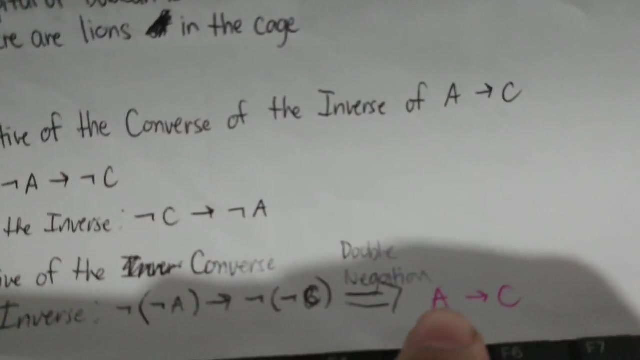 negation of C, Now applying the double negation law. in logic it's like negative times negative, you will have positive, negative times negative, you will have positive. So the contrapositive of the converse of the inverse of A implies C is just simply the original statement. 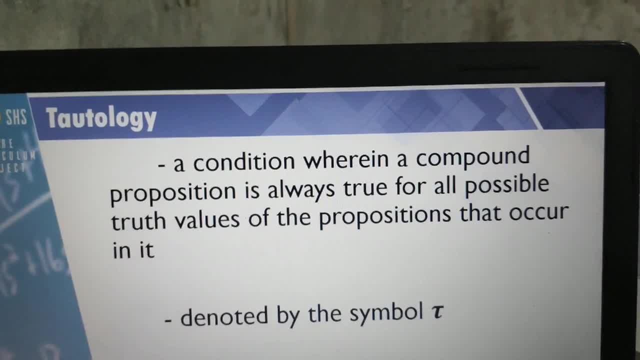 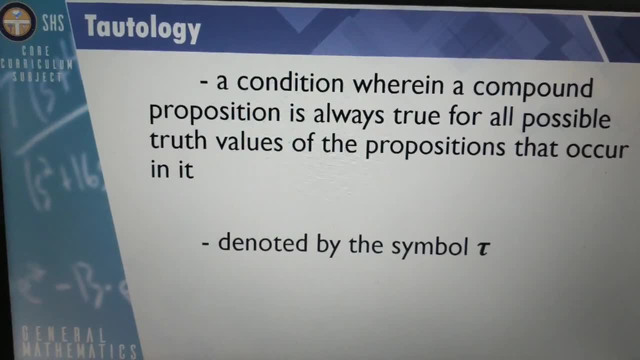 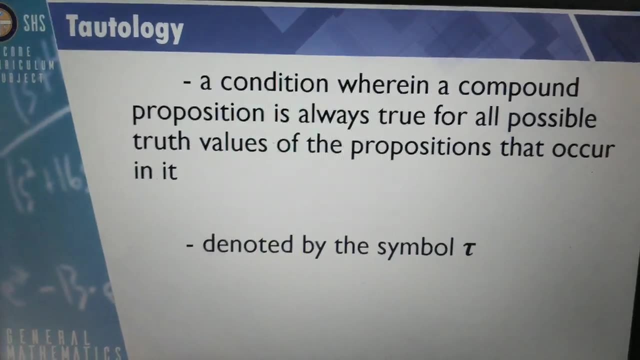 So we will now be moving to the actual lesson about tautology: contrapositive. So for a statement or for the compound proposition to be a tautology, the condition wherein a compound proposition is always true for all possible truth values of the proposition, that 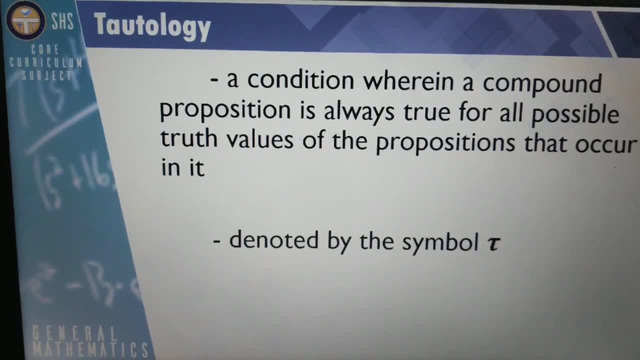 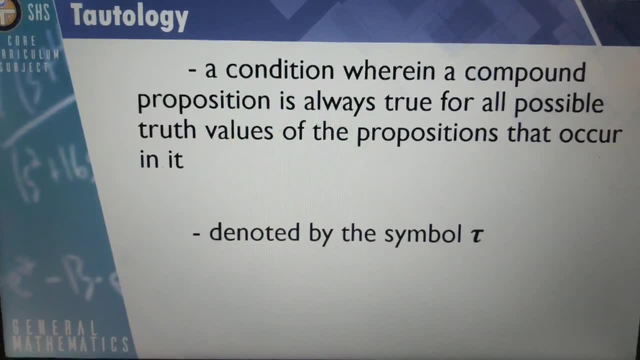 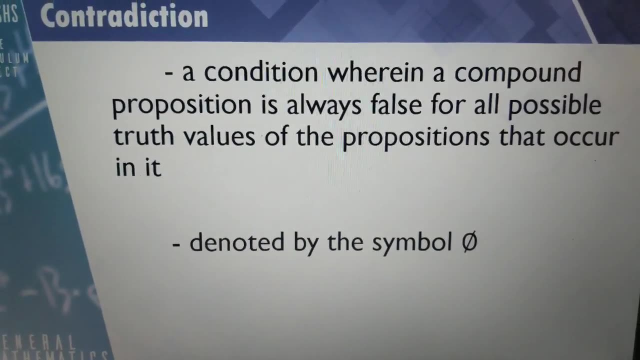 occur in it. Meaning, even if you consider for the different conditions of the compound propositions, it will always be true, The conclusion will always be true, So it will be denoted by the Greek symbol. Then you have the concept of contradiction. So it's a condition wherein a compound proposition 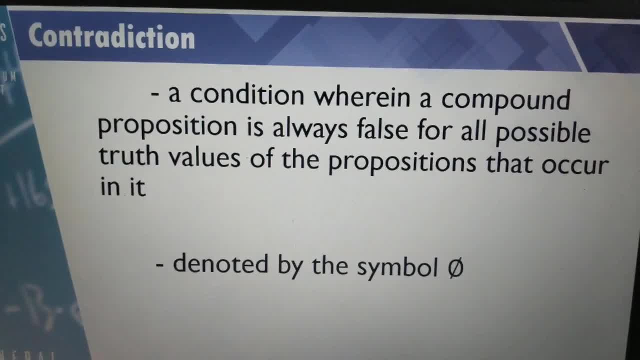 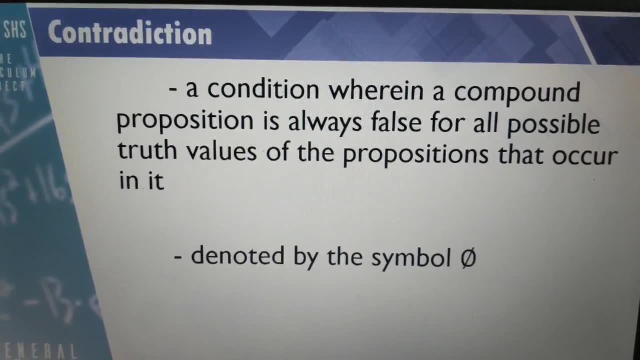 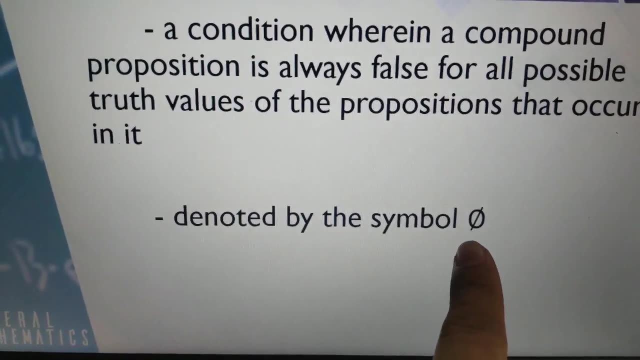 is always false for all possible truth values of the propositions that occur on it. So for the combination of different compound statements or compound propositions, the outcome would always be false And it will be denoted by the symbol: null set or no set at all. So 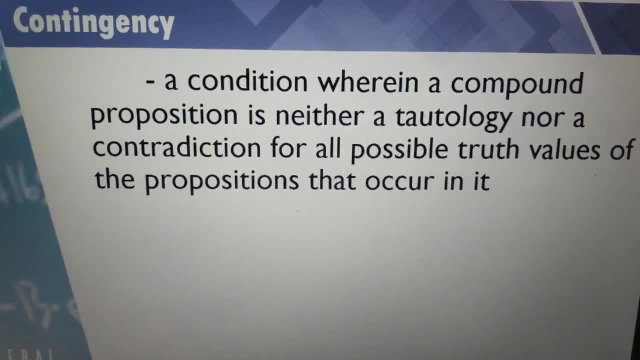 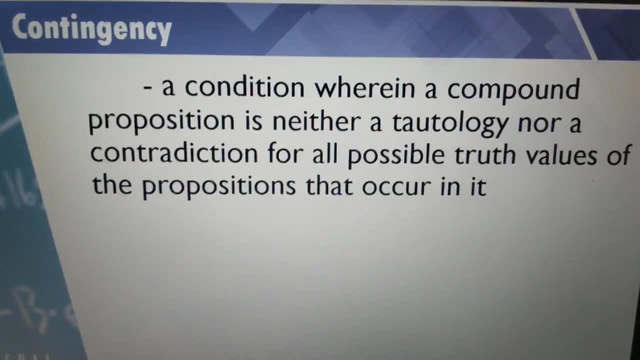 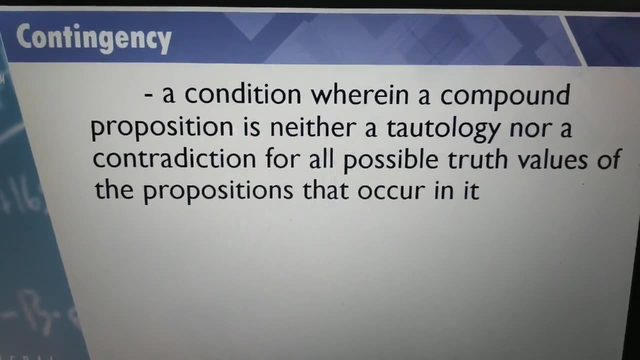 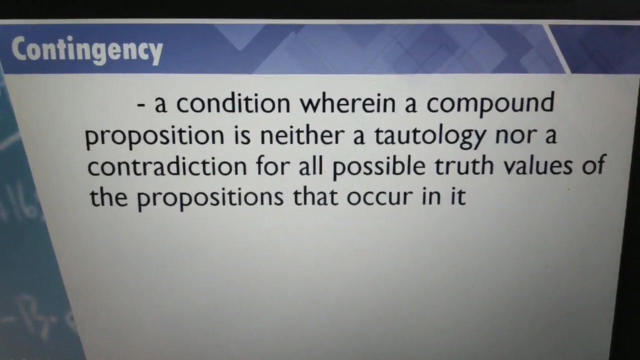 for the last, for the contingency, it's a condition wherein a compound proposition is neither a tautology nor a contradiction for all possible truth values of the propositions that occur on it. So meaning a statement or a compound proposition will be called contingency if the conclusion will have a mixed outcome of true and false. 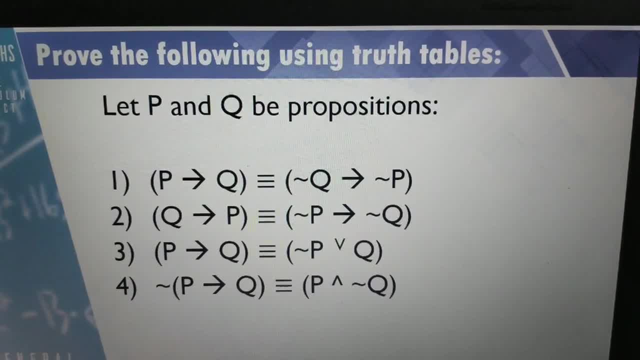 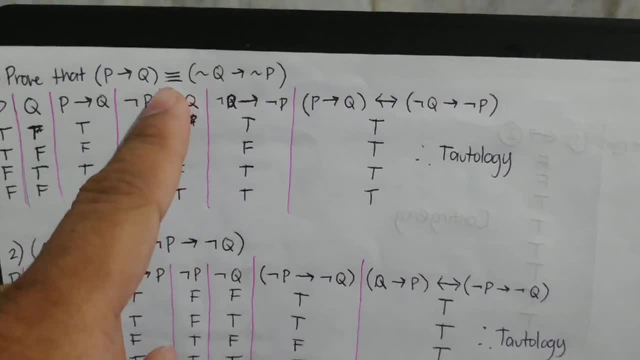 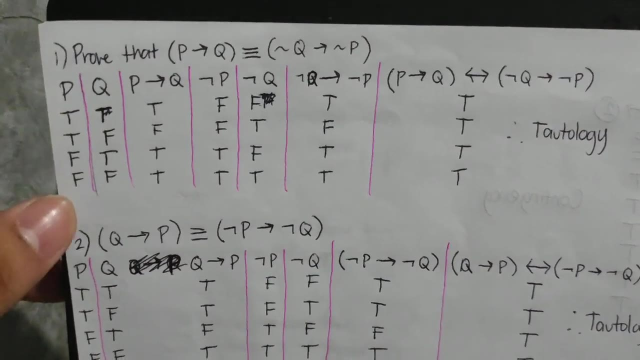 So let's prove the following using the Truth tables. So let's first prove that P implies Q is logically equivalent to negation of Q implies P. So, using the Truth tabels, we will consider all the possible conditions for the statements. 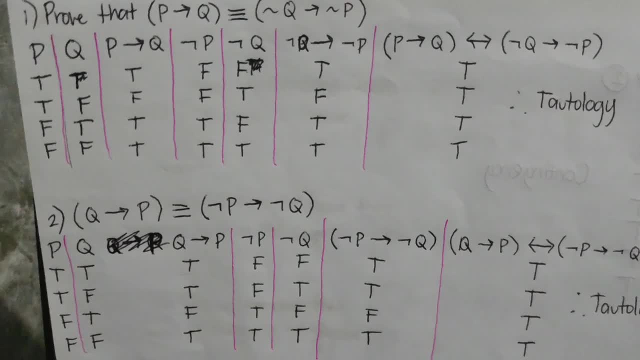 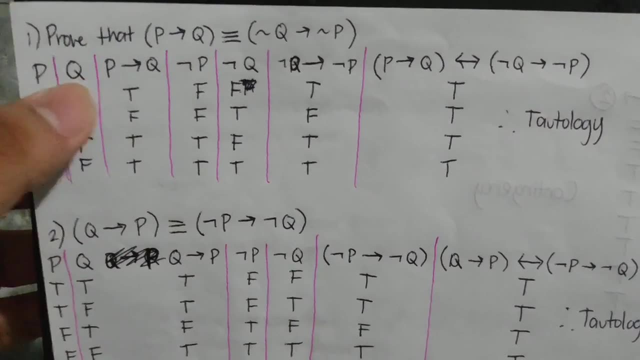 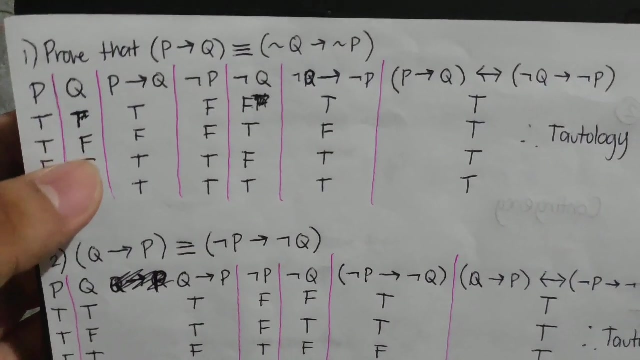 P and Q. If you have only one proposition, then you will have two conditions: that it will be true or false. since you have the statements P and Q, that is included for the the truth values, then you will have four conditions. you have true, true, true, false. 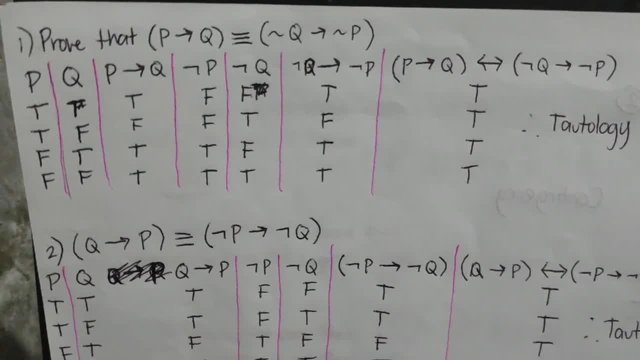 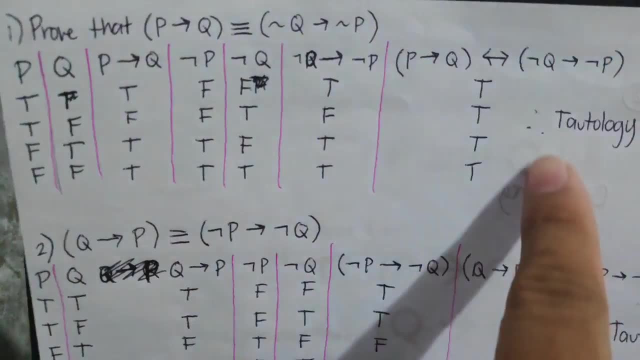 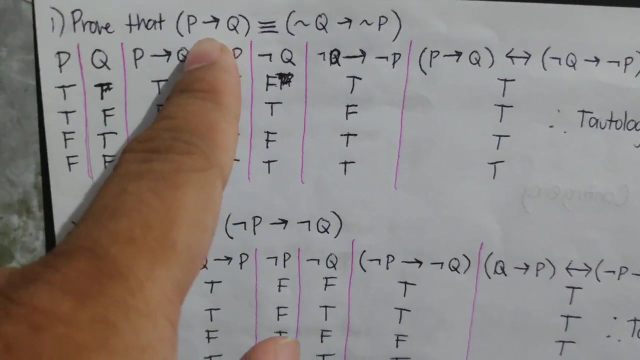 false, true and false, false. so we will be proving using the truth values. so our, our goal here is to find that the conclusion will be a tautology. so how did it become a tautology? so let's first consider the first condition or for the first compound statement you have: p implies q, so 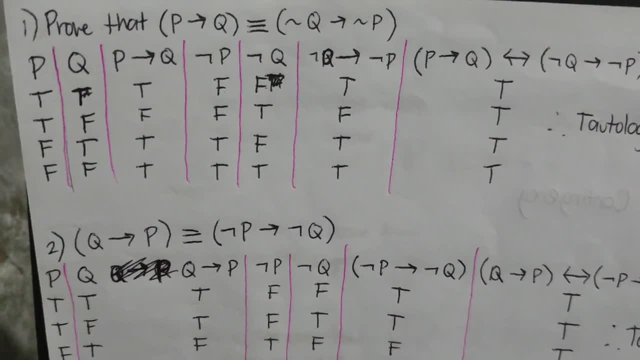 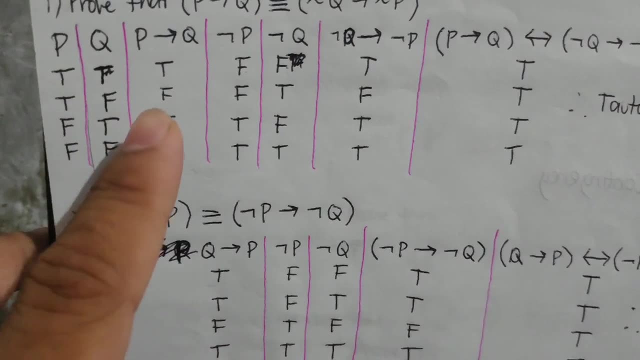 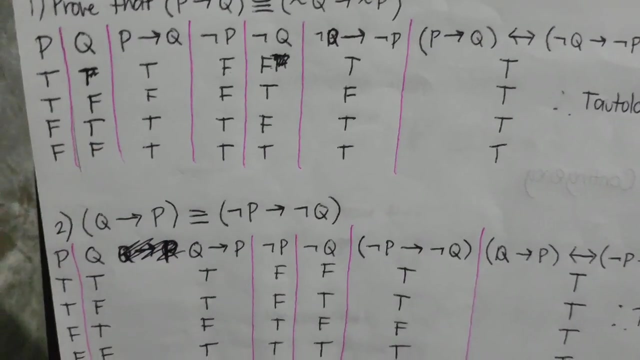 following the rules or the truth table for the compound proposition. conditional statement: if we have true and true, you will have true. true becomes false. therefore false, false then true that becomes true. false implies false then becomes true. so, since we are needing for the second part of our 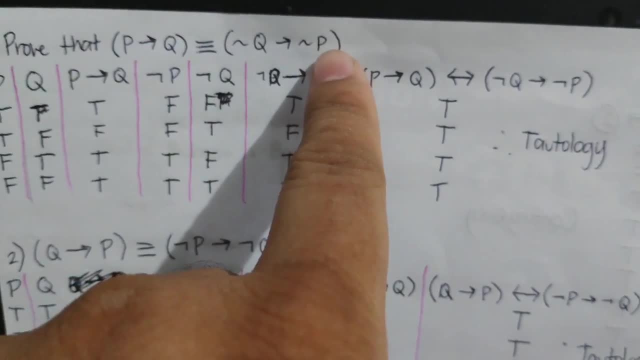 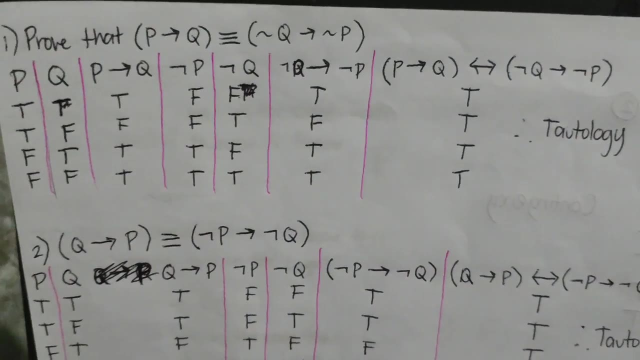 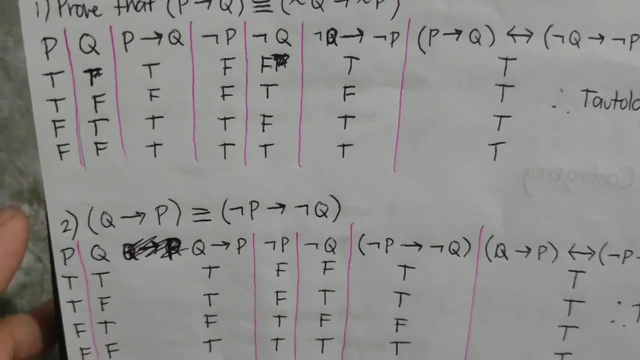 proving is, the negation of Q implies the negation of P. we need first to find the truth value of of the negation of p and the negation of q. So for the negation you will just only get the opposite truth value of each condition. So originally p is true, true, false, false therefore. 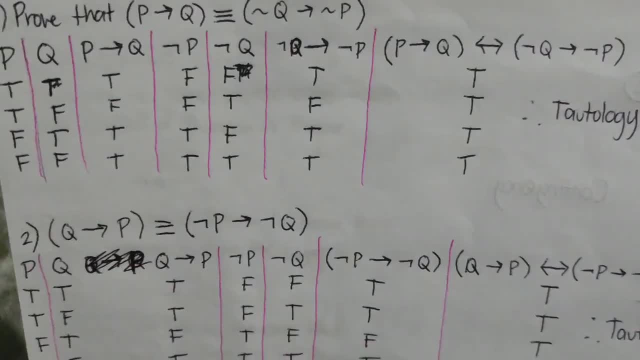 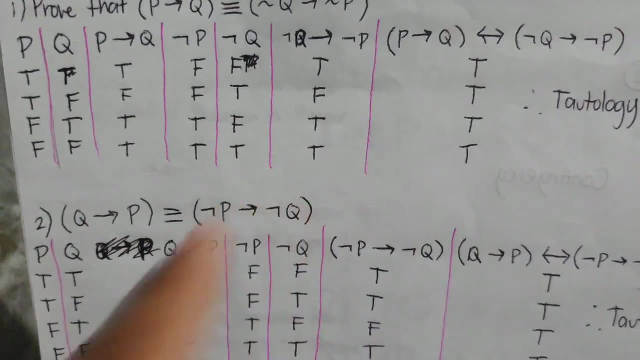 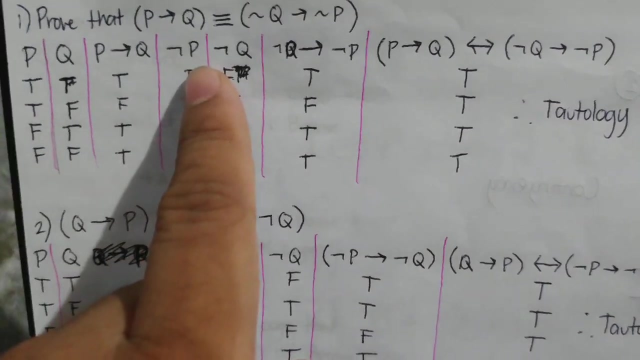 if you negate, it becomes false, false, true, true. and for q you have true, false, true, false. so negation will become false, true, false, false, Since we have successfully made the truth value for the negation of p and the negation of q. therefore, we can now find the truth value. 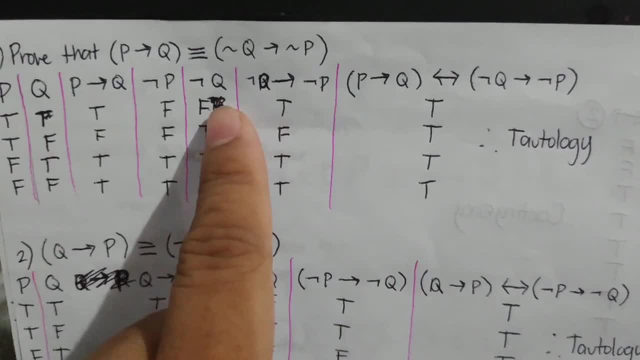 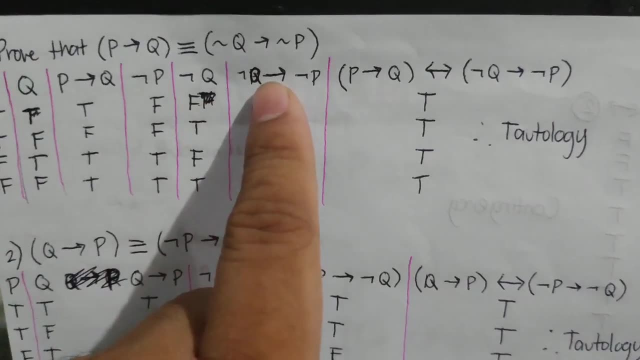 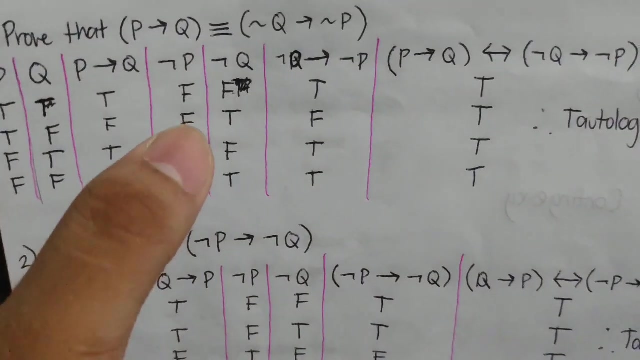 for the negation of q implies the negation of p, Since the conditional statement starts with the negation of q. so we will not go from left to right, but rather we will read the truth value from right to left, because that is the conditional statement. So you have: negation of q implies the 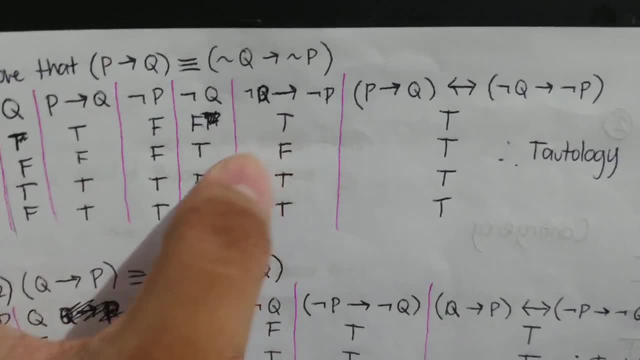 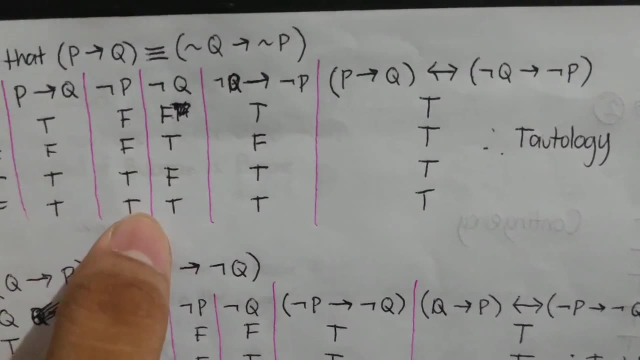 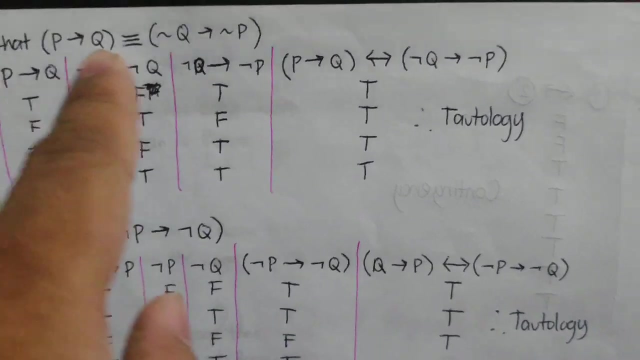 negation of p. so you have: f implies f, therefore true. True implies f, therefore true, Therefore false. false implies true, therefore true. so true implies true, therefore true. Now, since we have completed the conditions for the p implies q and the negation of q implies the negation of p. 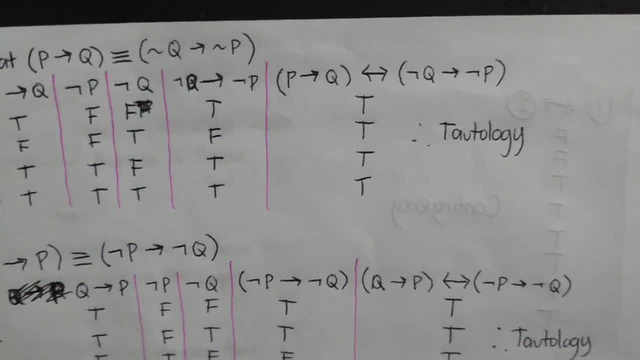 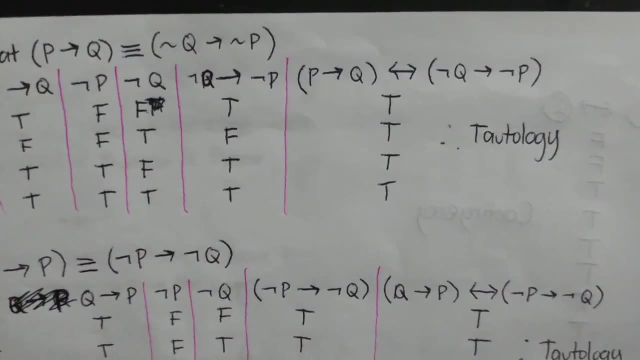 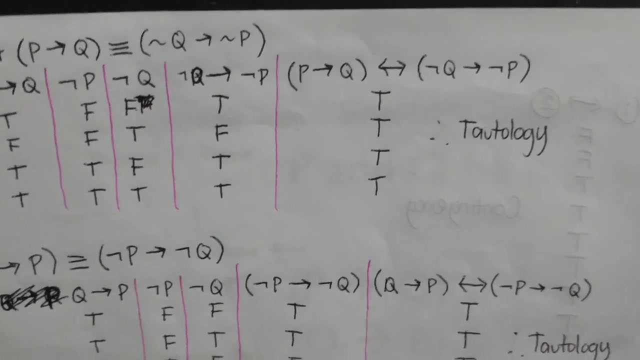 how are we going to prove that they are logically equivalent? Now, in logic, if two compound statements are logically equivalent, therefore they are biconditional. So we will prove the truth. value will always be true for it to be at tautology. So we will be looking here from p implies to q and 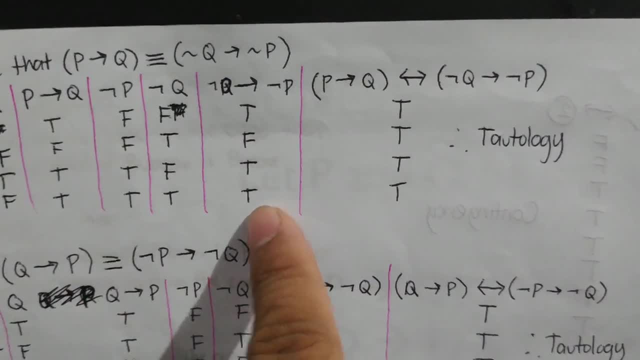 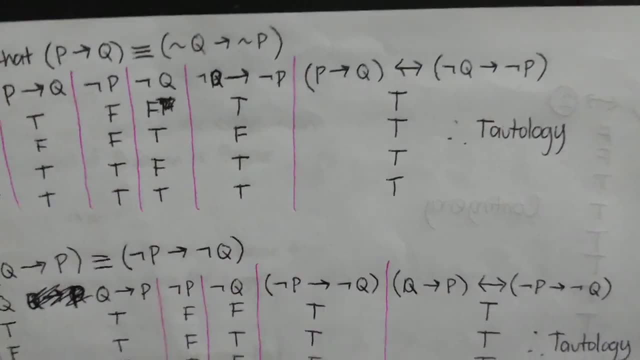 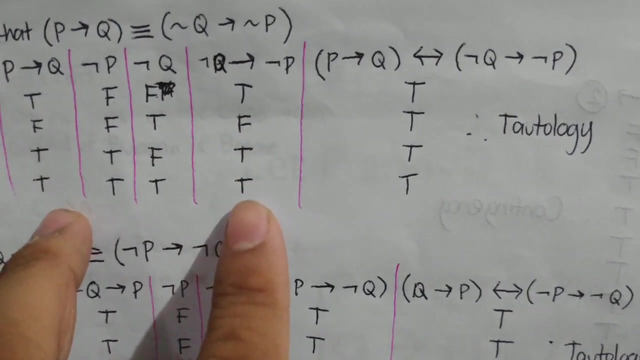 the truth value. from negation of q implies the negation of p. So the biconditional statement will always be true if the two truth values will be equal. So if we have here true and true, you will have true, false, false, true, true, true, true. then you have true and true. that means true. Now for 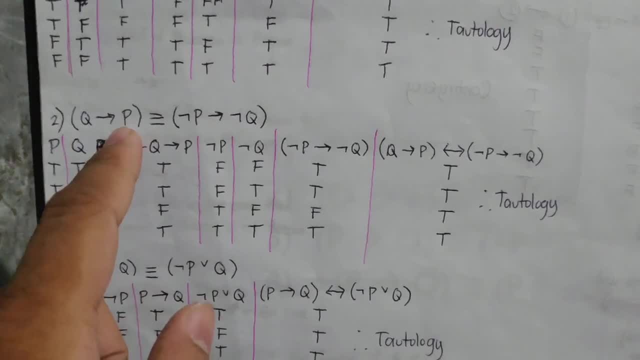 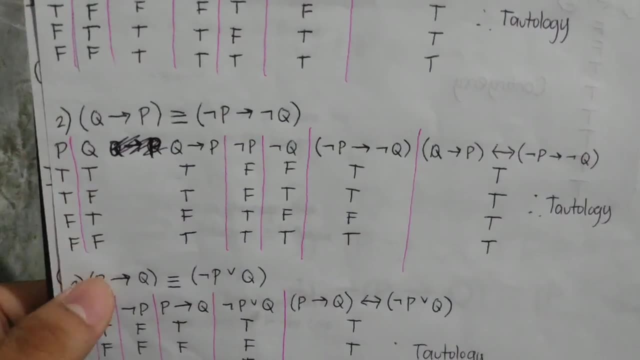 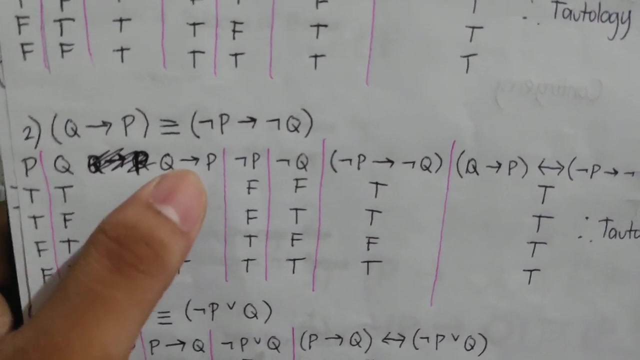 example, you have q implies p, it must be logically equivalent to negation of p and implies negation of q. So, following again the statements p and q, you have true, true, true, false, false, true, false, false. So we will start with: q implies p. so you have true, true, then true, false to true then becomes: 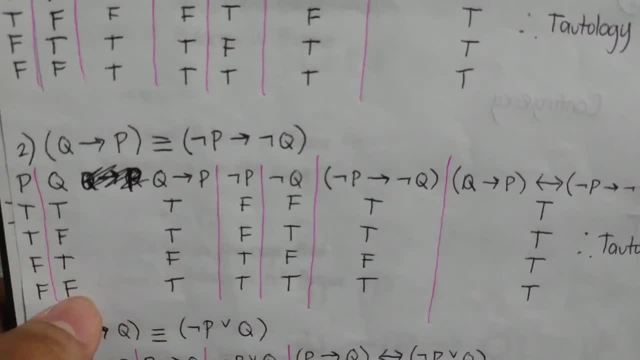 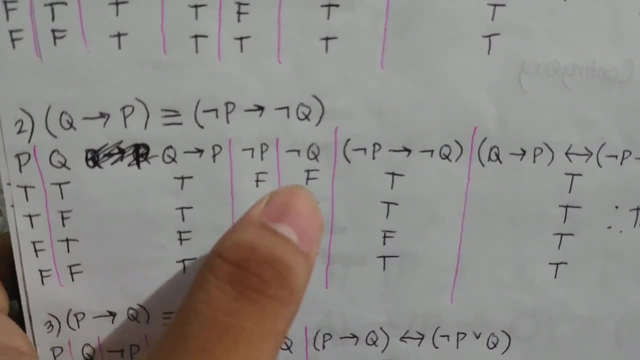 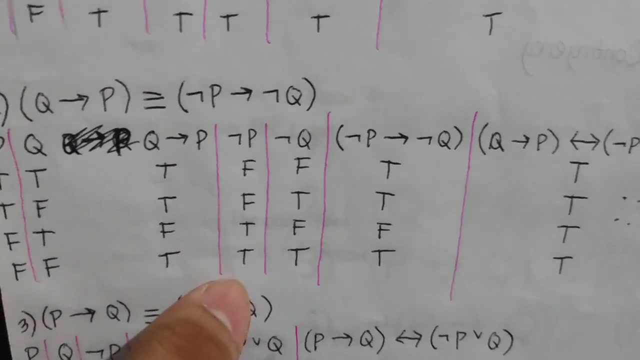 true, True becomes false, then becomes false. so false, false, it becomes true, True. then we get the negation of p and the negation of q, since it's vital for the compound proposition. So this becomes false, false, true, true. then for the negation of q, you have false, true. 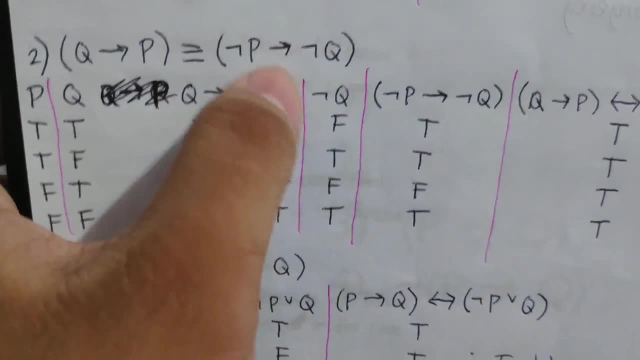 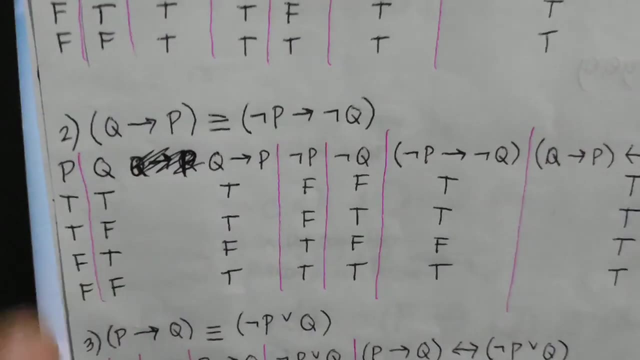 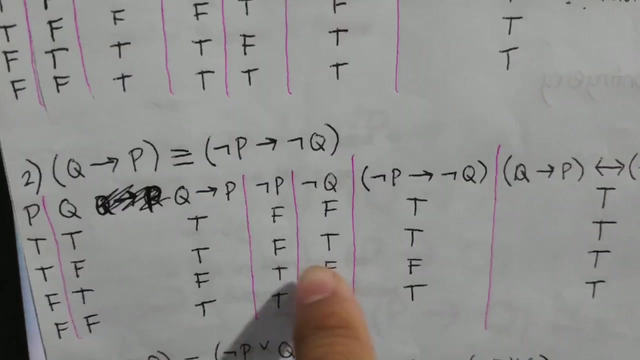 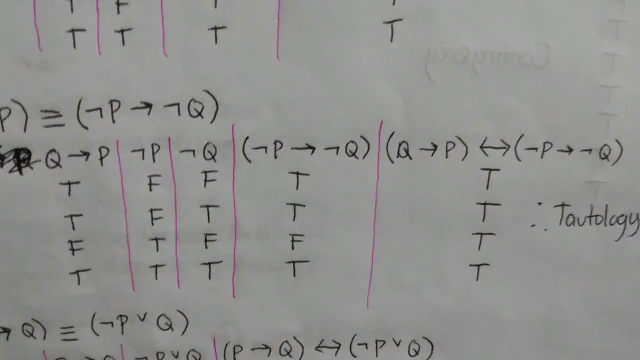 false, true. Then for the compound statement you will get now: the negation of p implies the negation of q, So we will now read it from left to right. So you have: false implies false. then for true, false implies true, therefore true. True implies false, therefore false. True implies true, therefore true, Since we have now the truth. 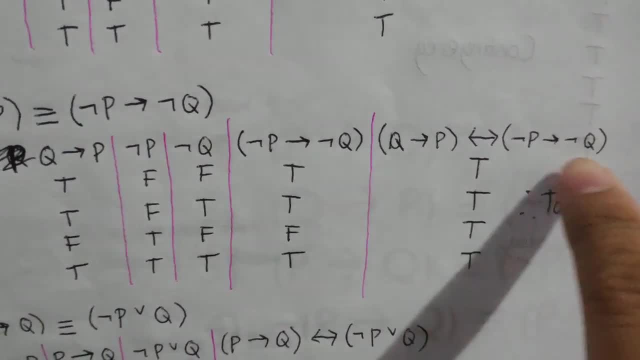 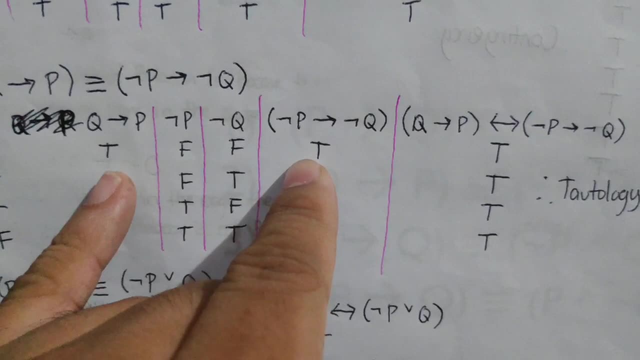 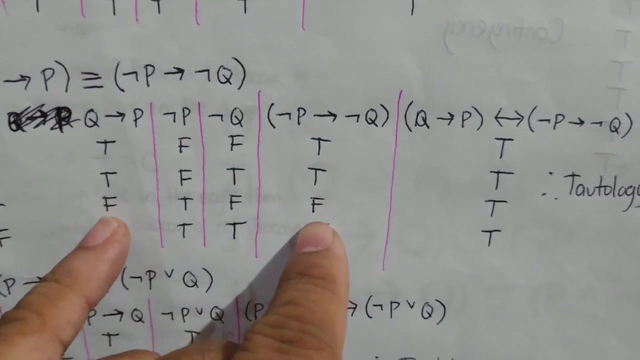 values, for q implies p and the negation of p implies q, we will now get their biconditional truth value. So again for the biconditional, they must have the same or equal truth value. So you have true: true, therefore true. True, true, therefore true. False: false therefore true. Then you have 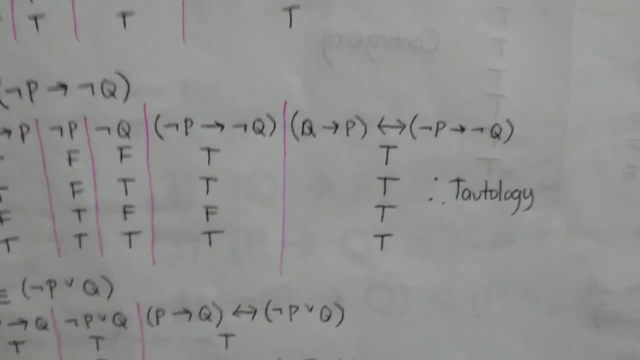 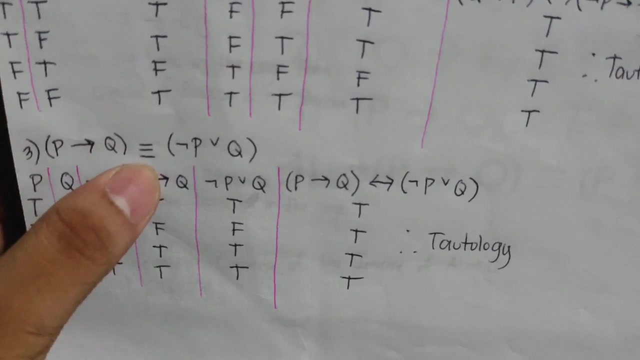 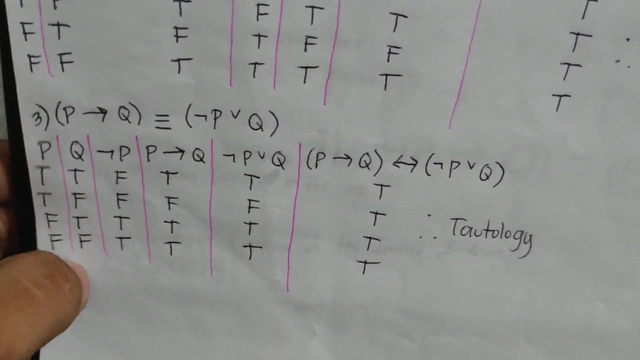 true, therefore true. So for number two, you have also the tautology. Now for number three, you have p implies q, which is logically equivalent to the negation of p or statement q. So again write the truth values for the initial primitive propositions. We have p and q, so it is vital. 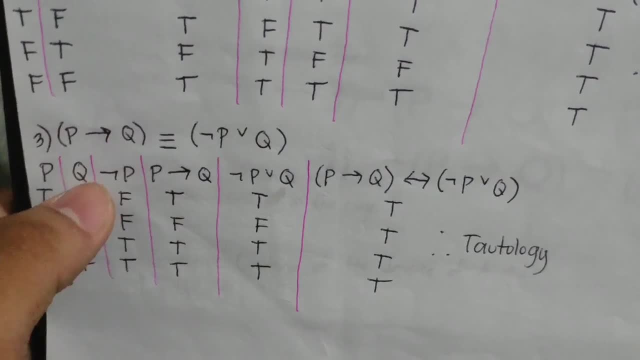 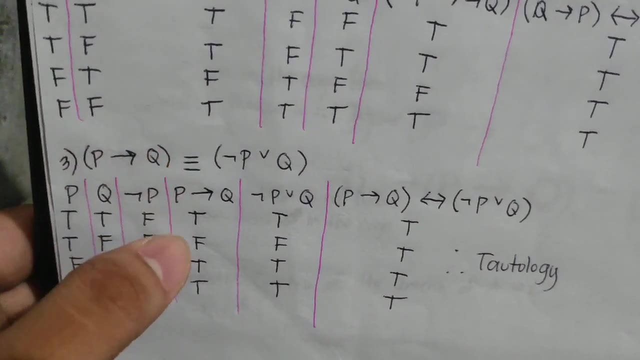 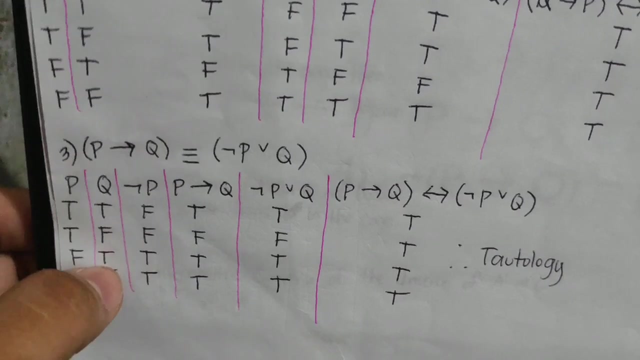 that we need the negation of p, therefore the truth value for the negation of p, provided column. then you have p implies q. so you will look at the primitive propositions: true, true, therefore true, true, false, false, false, true, true, false, false, therefore true. and then you will have: 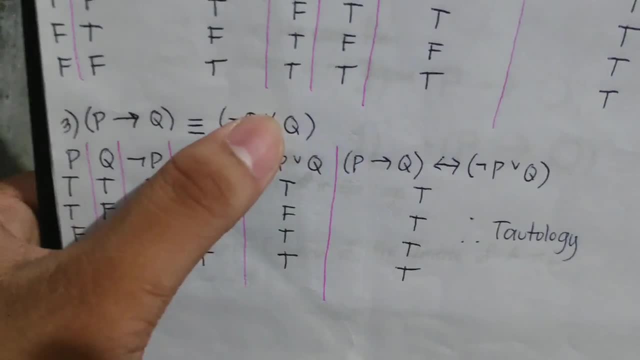 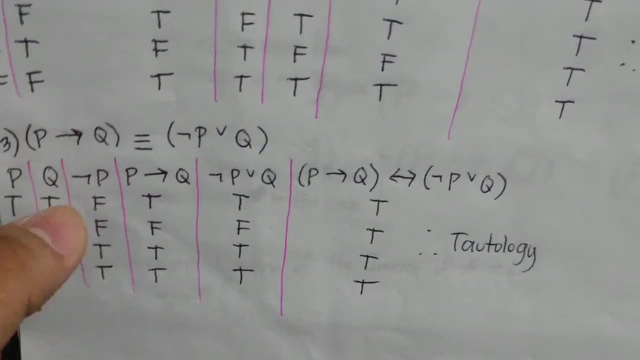 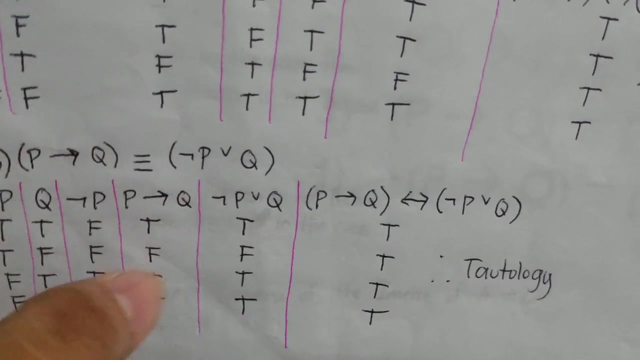 the disjunction of negation of p or q. so this is the disjunction. therefore, for the third value, for it to be true, one of the statements must also be true. so you have negation of p or q, you have false or true, therefore true. false or false, therefore false. true or true, therefore true. 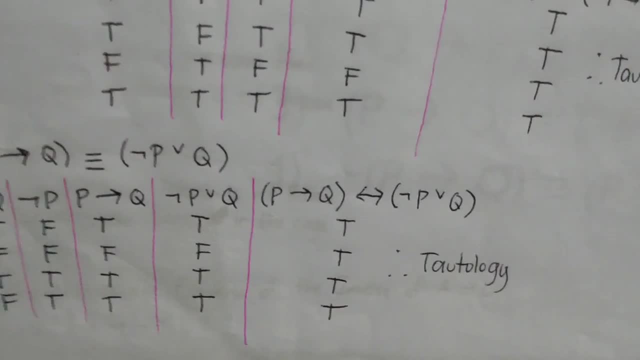 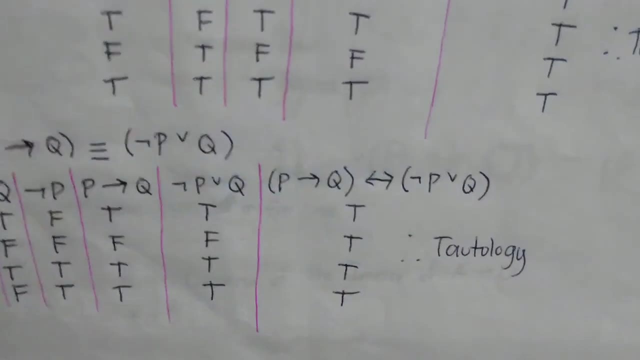 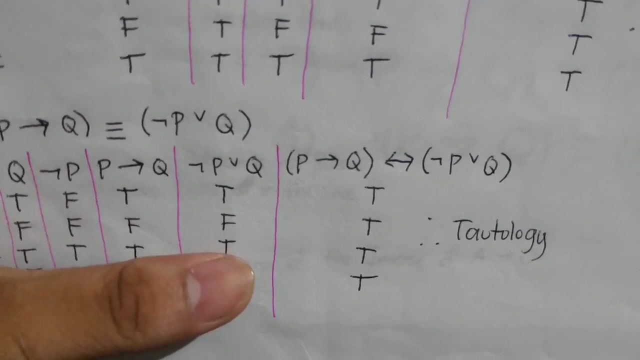 true or false, therefore true. since you have now the truth values, for p implies q and the negation of p or q, you will have the biconditional statement. so they must be equal: true. true therefore true. true, false, false, therefore true. true, true therefore true. and then for true and: 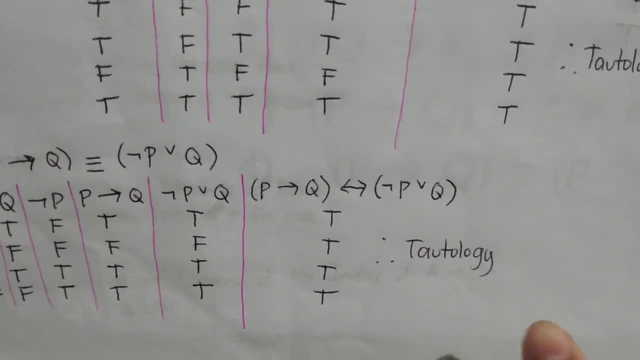 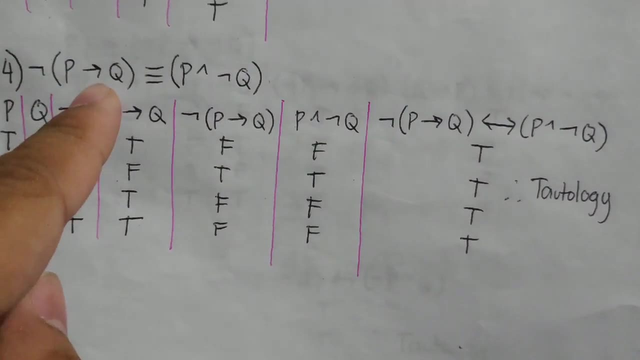 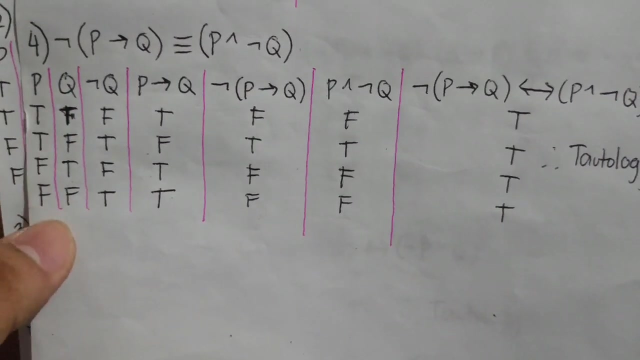 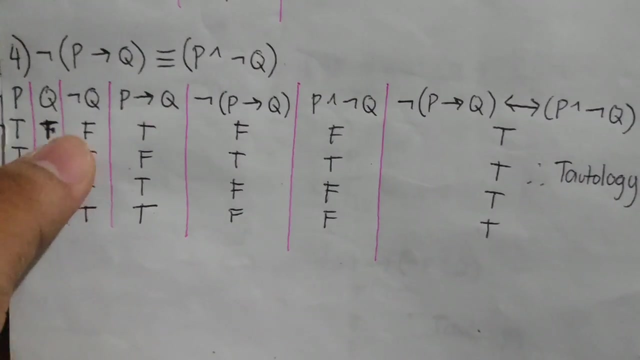 therefore true. so number three is also an example of a tau tau. and for the last example you will have, the negation of p implies q is logically equivalent to p and negation of q. so again, start with the initial truth values for the true two primitive propositions. now, this time we will be needing the negation of q, so you have. 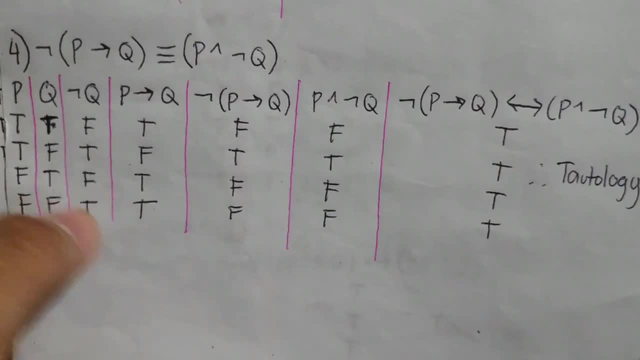 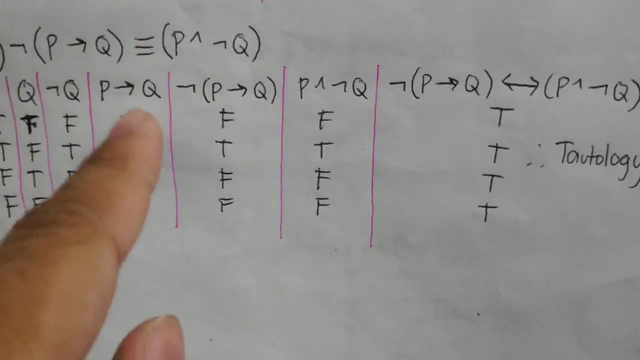 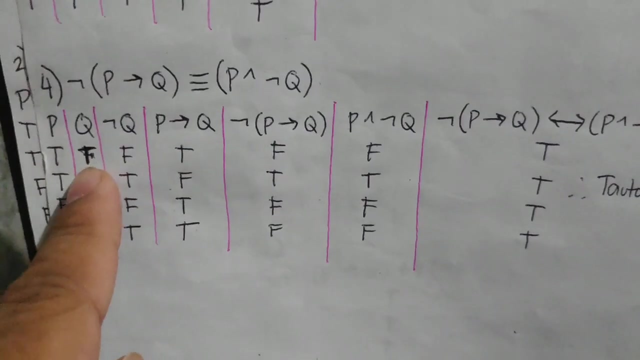 false, true, false, true, because you will be getting the opposite truth value for the statement q, then we will be needing first, before you negate the p implies q. you need the truth value for p implies q, so you have true, true. therefore, true, true, false, false, false, true, true, false, false true. 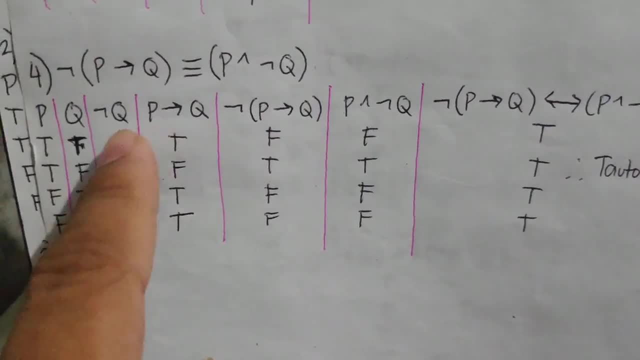 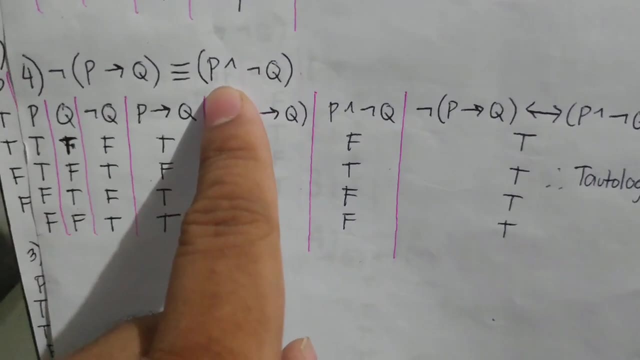 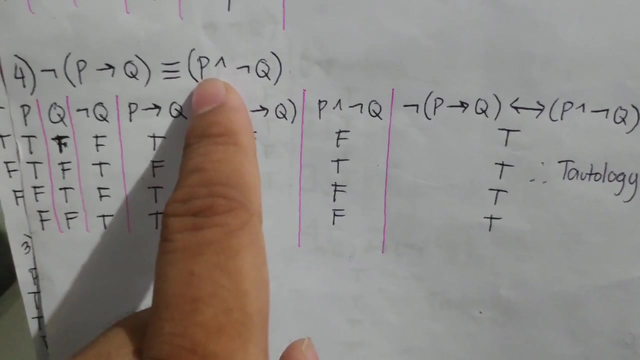 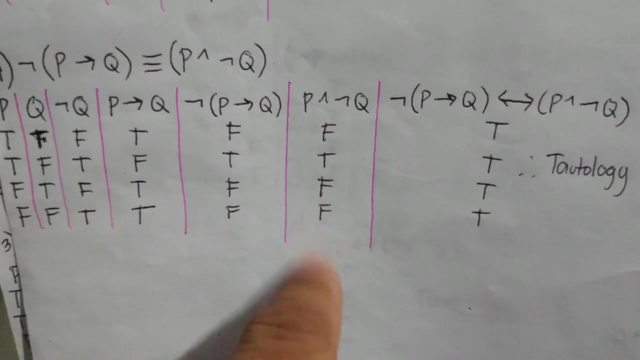 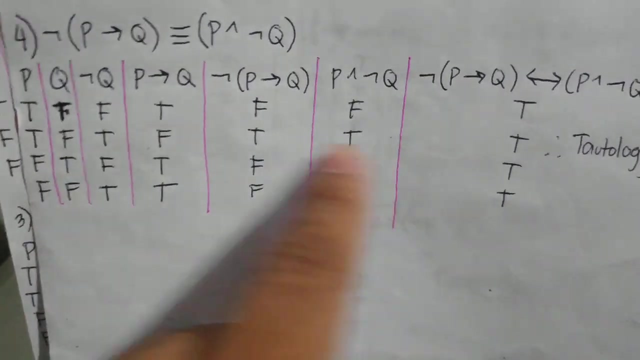 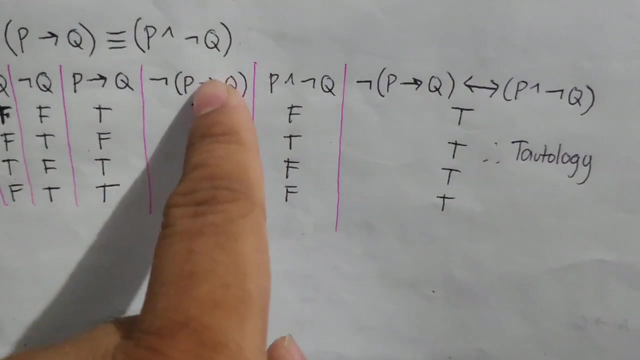 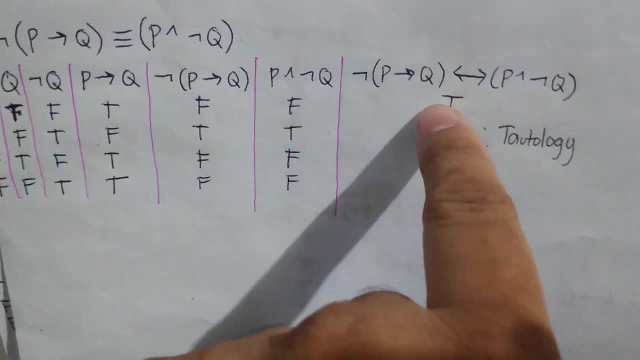 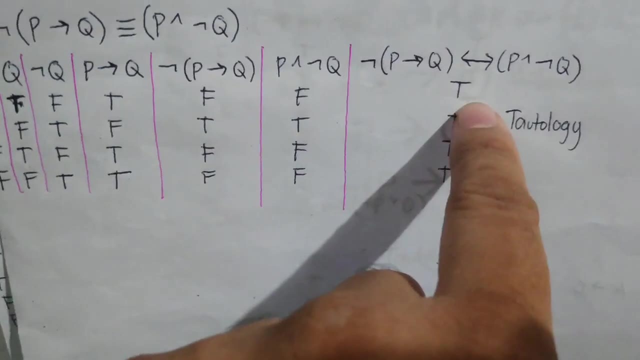 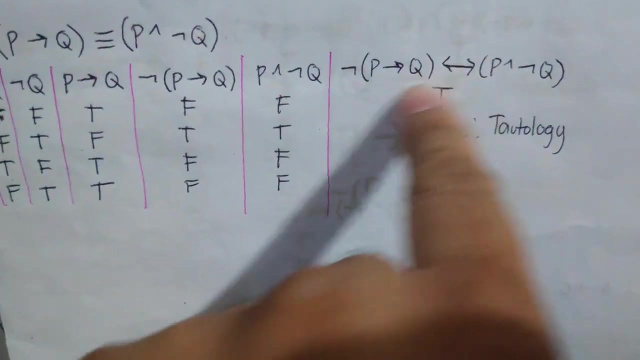 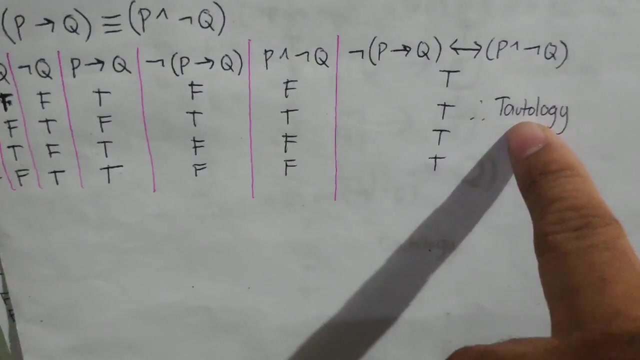 q. so we will see if there are logical equivalent, if the truth value for their biconditional statements will all be true. so by checking them, so false, false, you have true, true, true, therefore true, false, false, therefore true, false, false, therefore true. so the biconditional statement of these two compound propositions will have true for all conditions. therefore, statement number four, or logical equivalence number four, is also a. 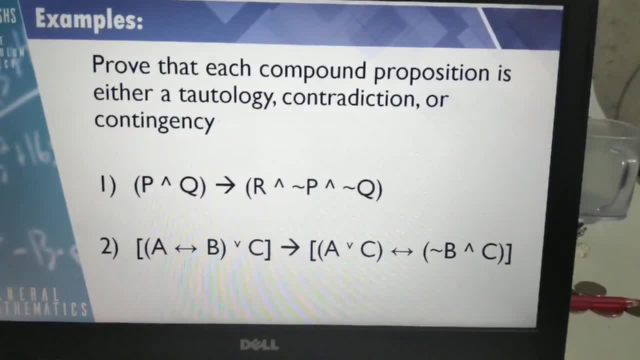 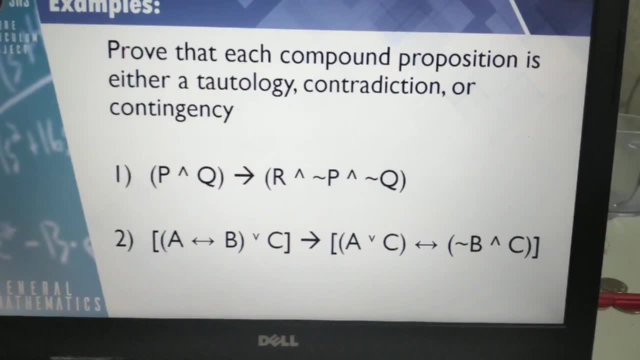 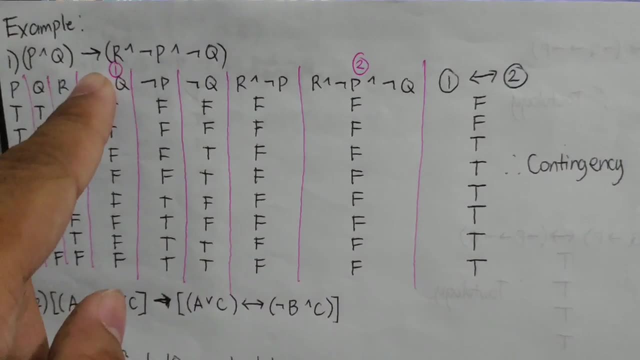 tautology. now for the last examples. you need to prove that each compound proposition is either a tautology, a contradiction or contingency. so let's start first with number. so for number one you have p, and q implies r and the negation of p and the negation of q. 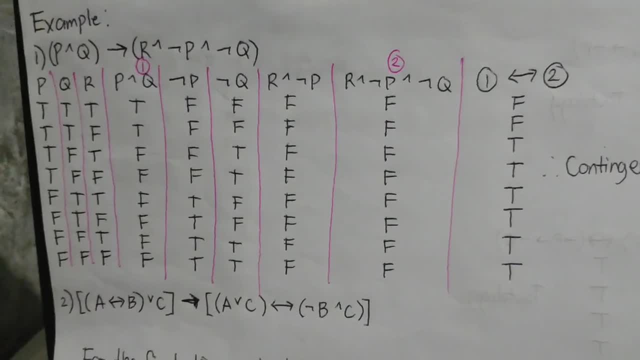 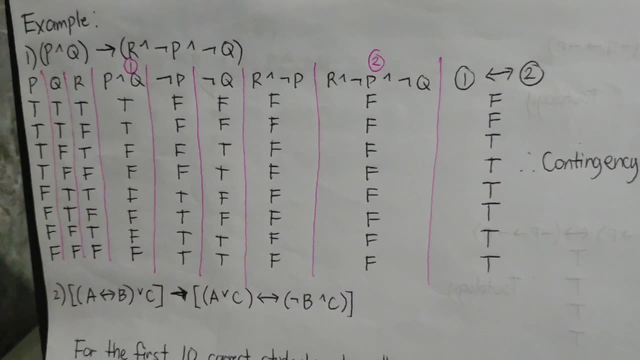 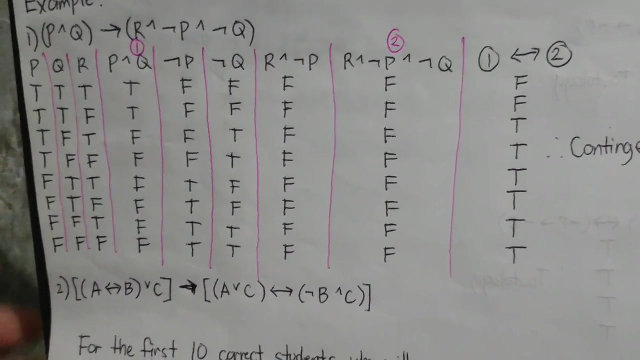 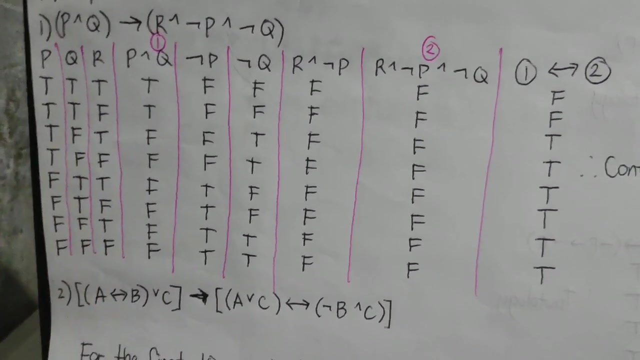 so you will be dealing with three primitive propositions. earlier we have only discussed about two propositions, so it will only be good for four possible conditions. since you have three conditions or three propositions, the conditions will now become eight. so these are all the possible conditions in which three propositions will be included. so for p, you have four. true, 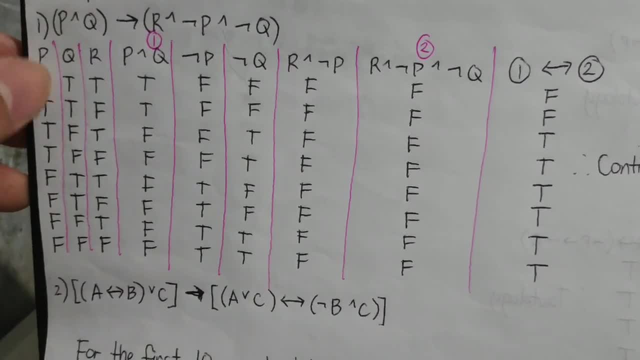 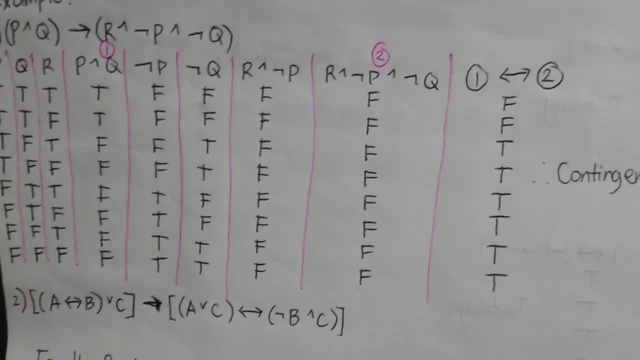 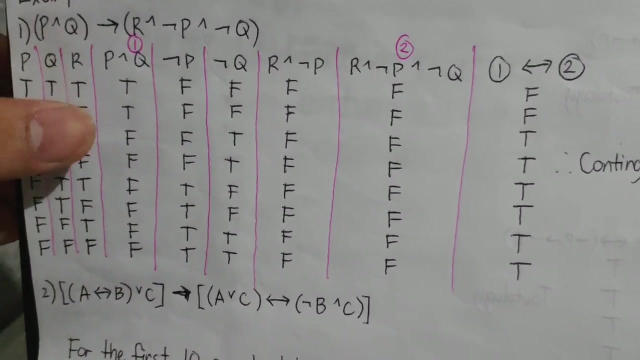 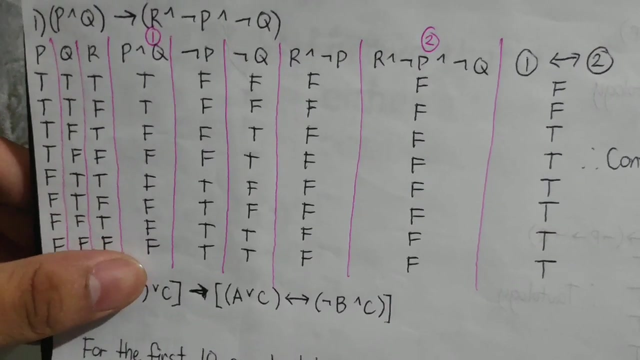 four, false, four q, same number, but with alternating patterns. so you have true, true, false, false, true, true, false, false, and for the last proposition you will have an alternating result. so true, false, true, false, true, false, false. therefore, the eight possible conditions for the three propositions will be completed. now, for the first part or the 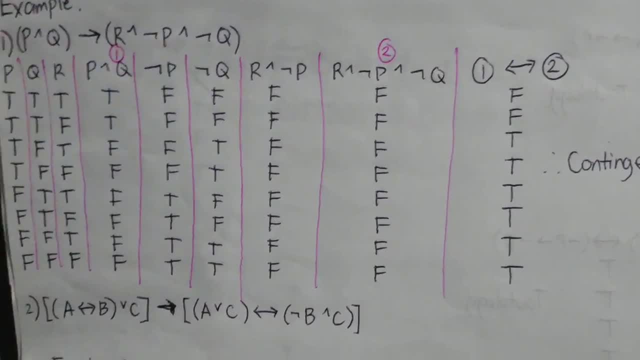 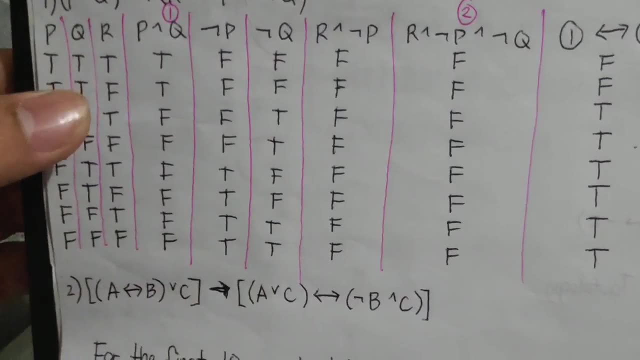 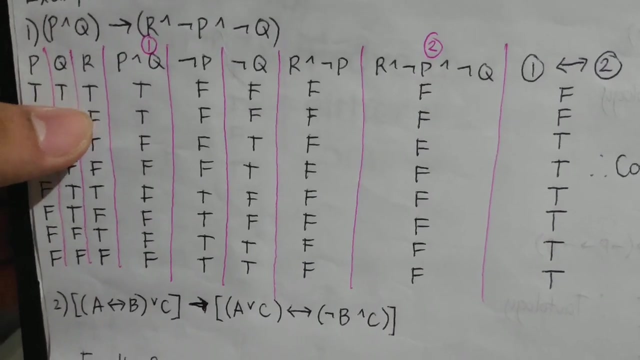 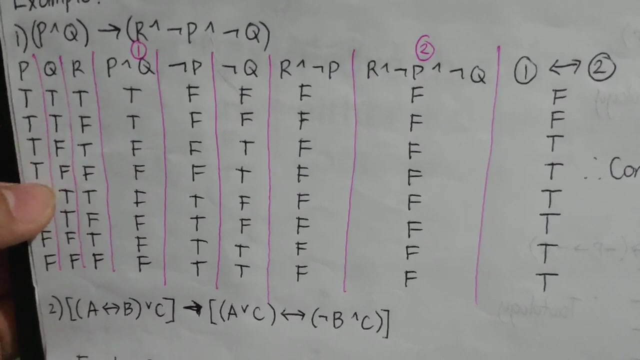 left side of the proving, we have p and q, so therefore we will have the conjunction of p and q. so they were the conjunction, will always only be true, will only be true if both compound or primitive propositions will have the same truth value. so you have true and true, therefore, true to true, therefore, through true and false, false true. 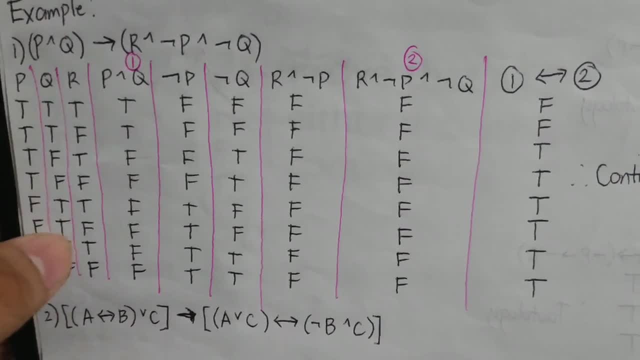 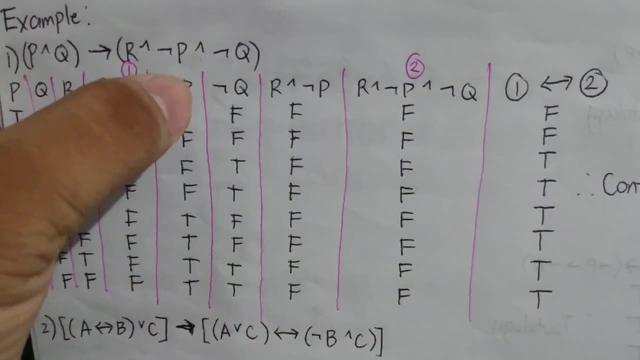 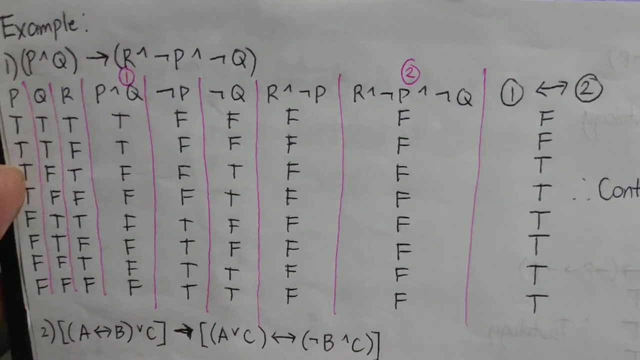 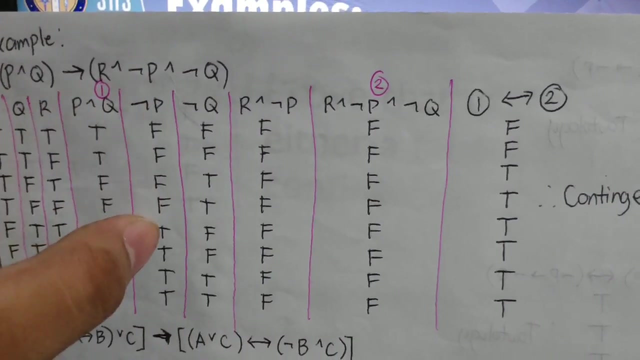 and false, false, false and true, false, false and true, false, false, false, false, false and false, therefore false. now we need the negation of P you p for the second part of our proving. so therefore, the fourth true and the fourth false will be negated. so this becomes for false and then for true. then we will. 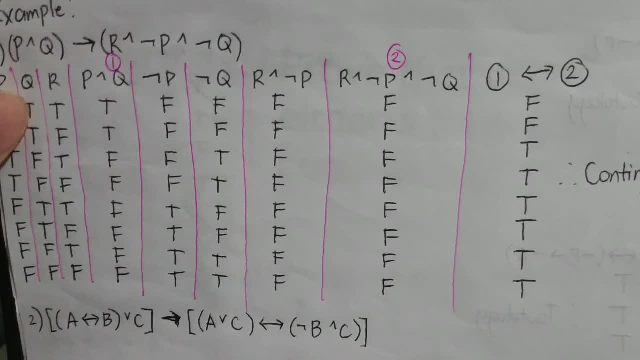 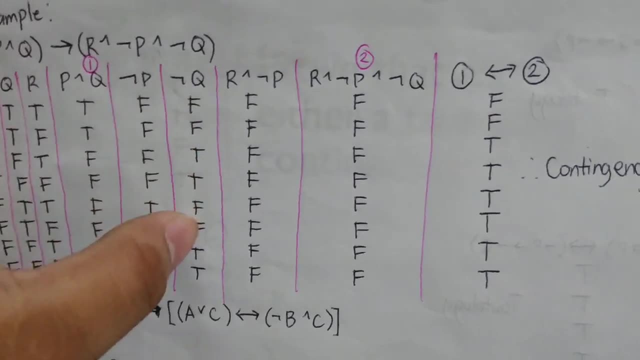 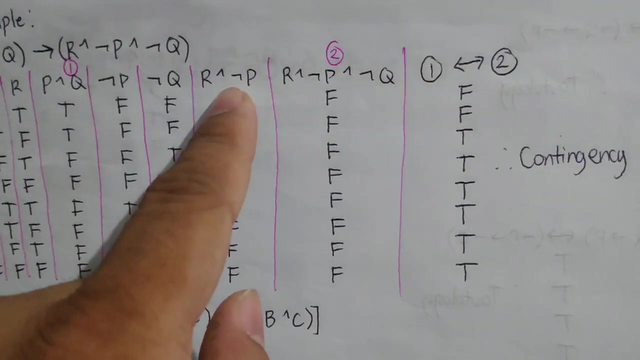 be having the negation of Q. so if you have the alternating true and false, that will start. for true, so it. for the negation of Q, it becomes false, false, true, true, false, false, true, true. then for the second part you still need to get the conjunction of R and the negation of P, so again for them to be. 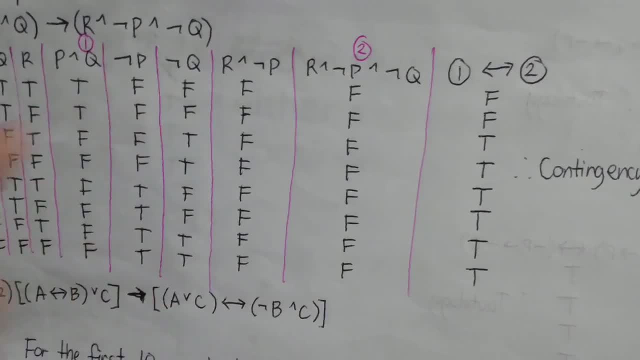 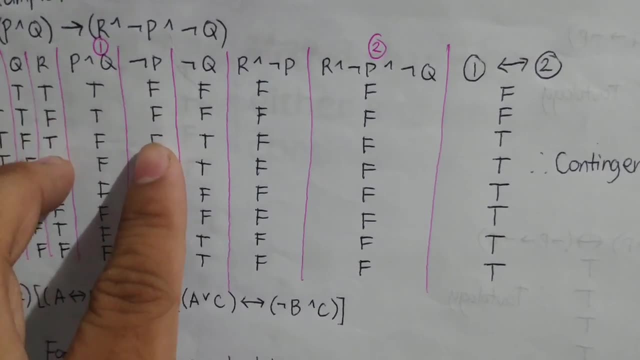 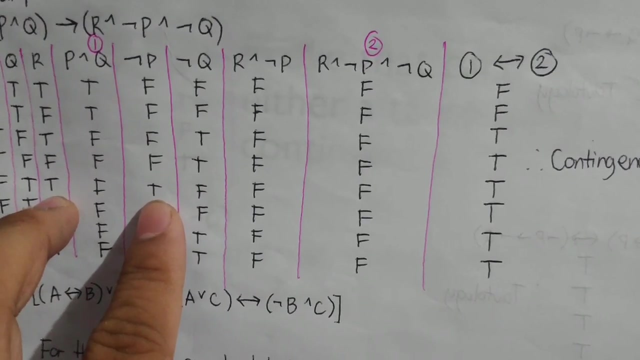 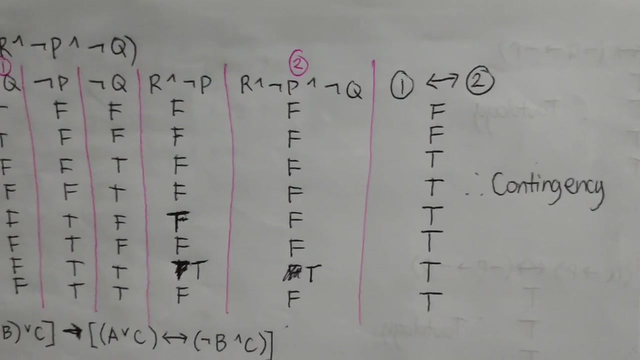 true, R and the negation of P would would need to be both true, so you have true, false, therefore false, false, false, false, true or false, false, false and false, false, true and true, therefore true, false and true. so we'll be having R and negation of P, negation of Q. 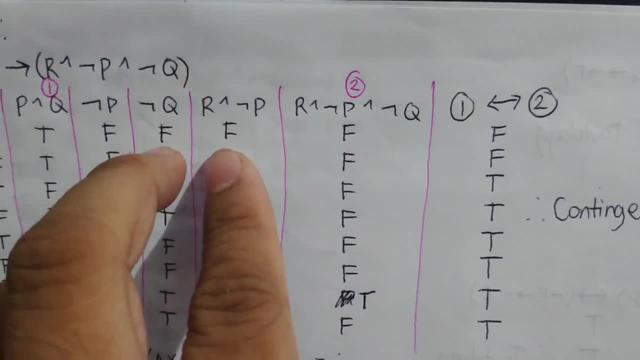 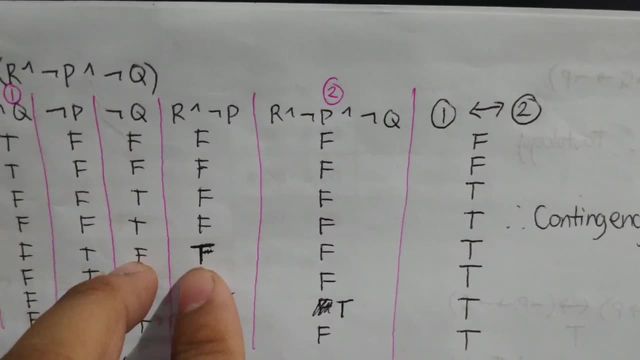 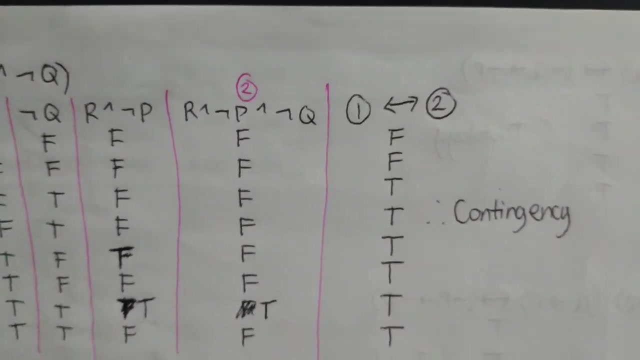 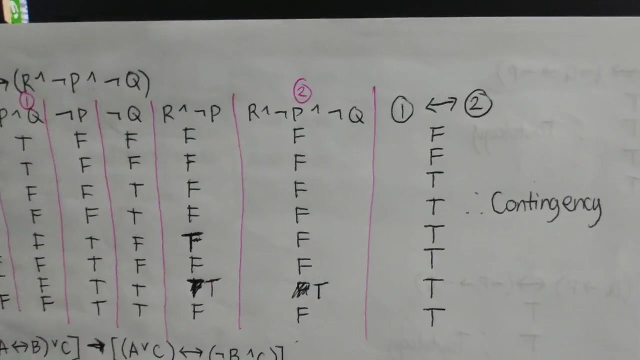 so we will be using this table and this table, so you have false, false, false, false, false, false, true, false, false, true, false, false, true, false, true, false, false, false, false, true and true, therefore, true, true, false, false, excuse me. and now a to get now the implication. so so we will be getting the implication of the first statement. 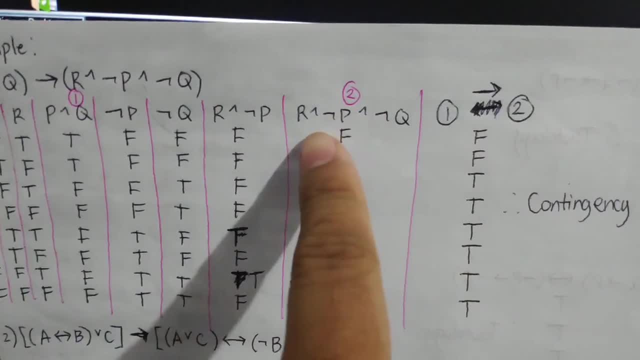 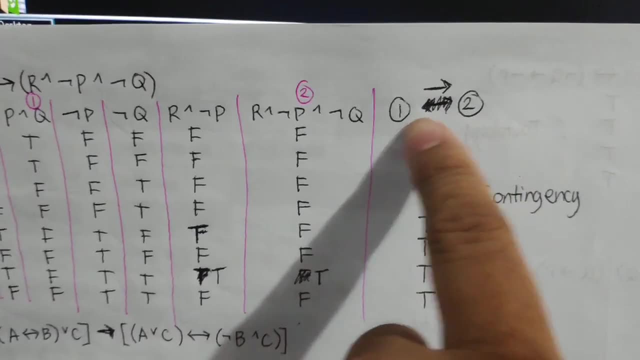 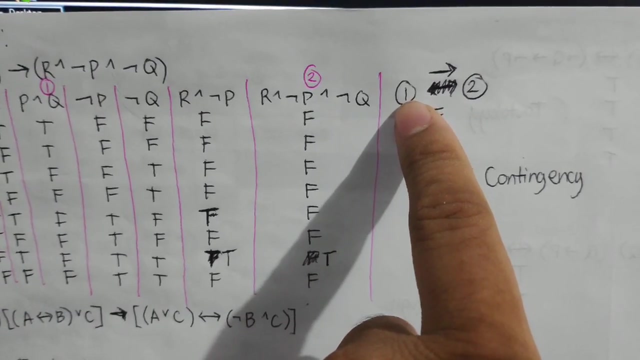 which is p and q, and then implying statement two, which is r, and negation of p and negation of q. so to avoid confusion for long writing of statements you can use numbers to symbolize with what proposition are you getting to. so if you have statement one, implies statement two. 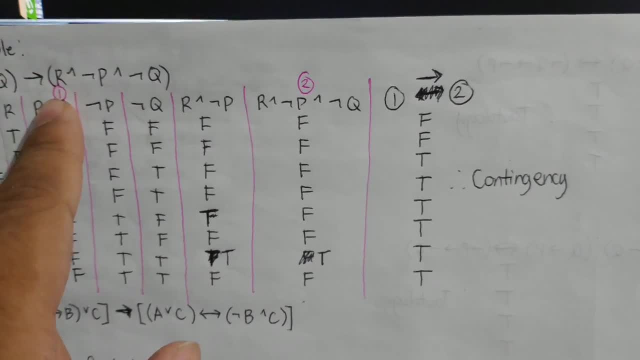 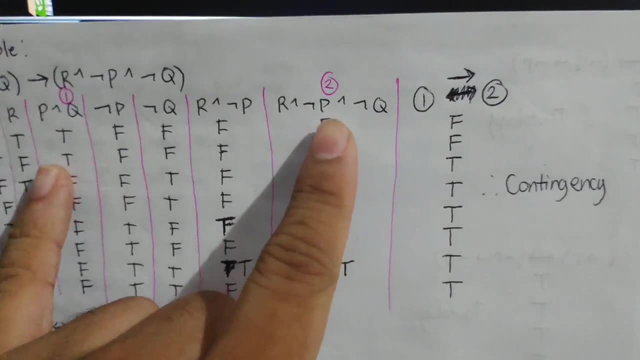 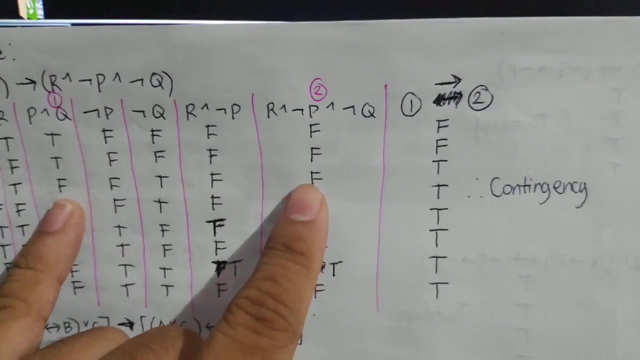 so you will apply here: p and q become statements one, and statement one rather and r and negation of p, negation of q will be statement two. so if you have the implication, so you have. true and true becomes false, therefore false. true becomes false, therefore false, false becomes false, therefore. 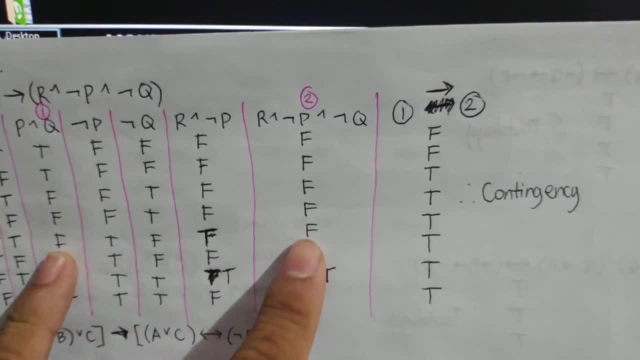 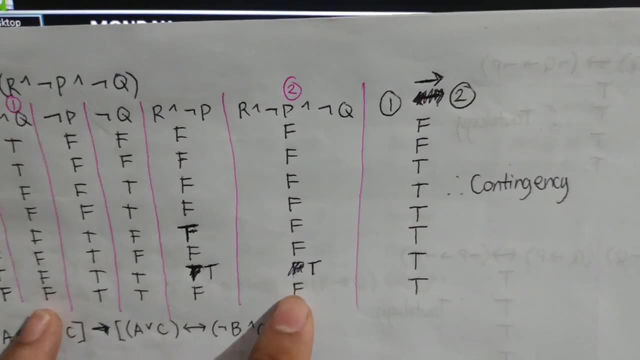 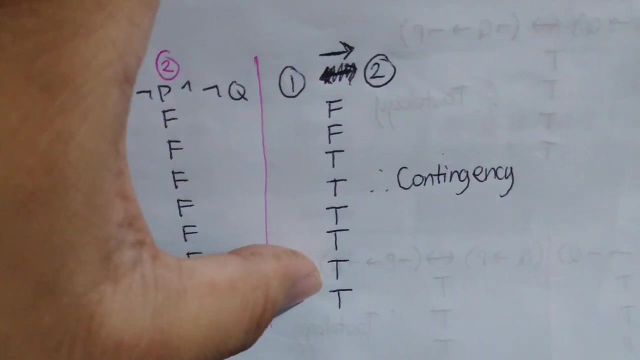 true. false becomes false, therefore true. false becomes false, therefore true. false becomes false, becomes true. false becomes true, therefore true. and then you have the last: false becomes false, therefore true. so here you could see that it almost became a tautology, but since you have the first two conditions to be false, so it's neither a tautology nor a. 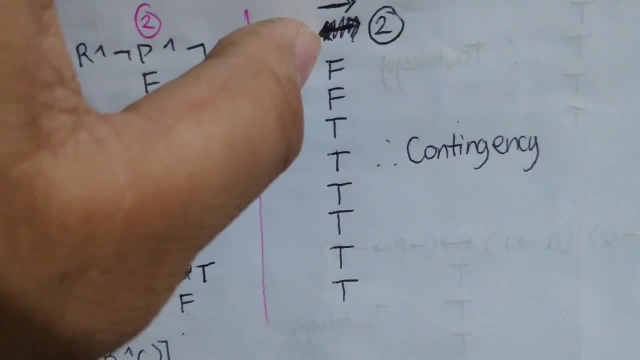 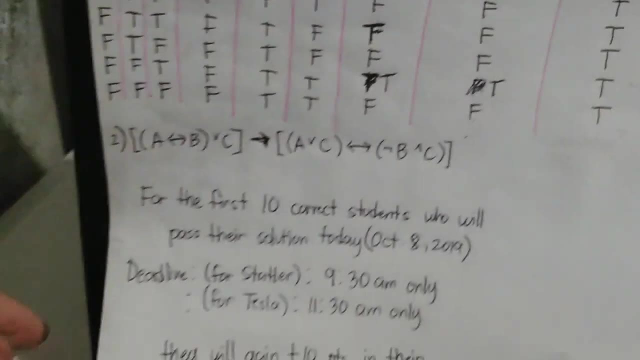 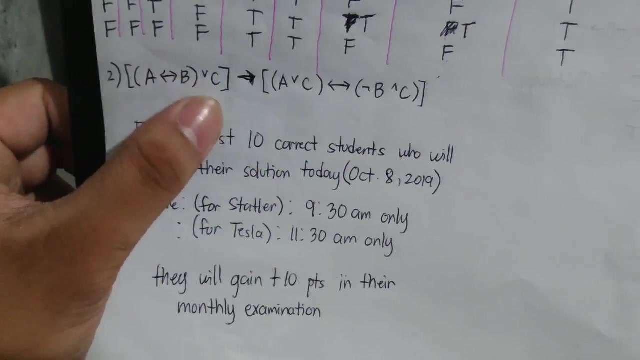 contradiction, because it is not all false. so you have the mixed possibilities of false and true. therefore, this is an example of a contingency. so for number two you have the statement a implies or, but it's biconditional to b or c implies that you have the biconditional for a or c. and 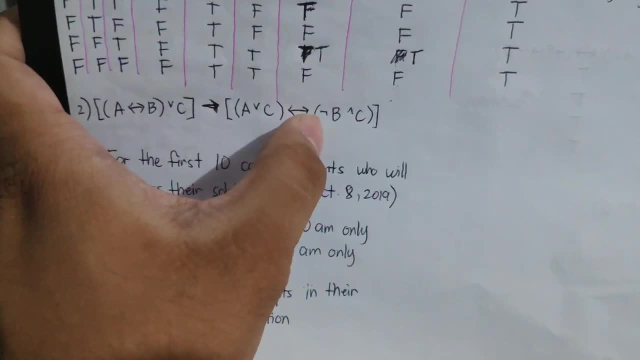 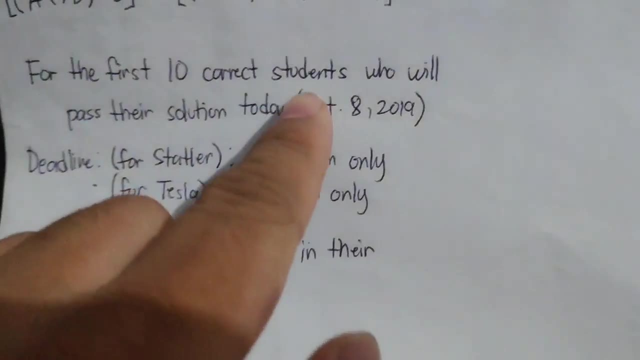 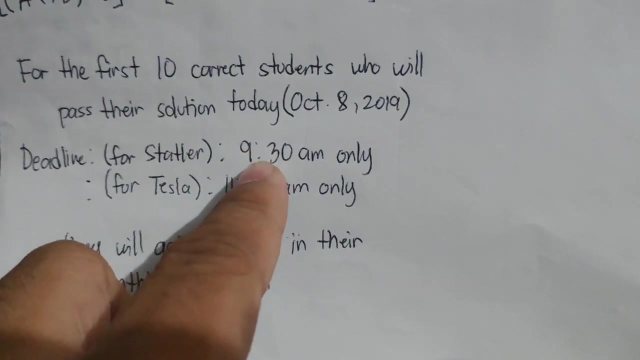 the biconditional if and only if, negation of p and c. so for the first 10 correct students who will pass their solution today, on october 8, 2019, you have the deadline. for statler, you have only until 9, 30 am to pass, and for tesla, you have only. 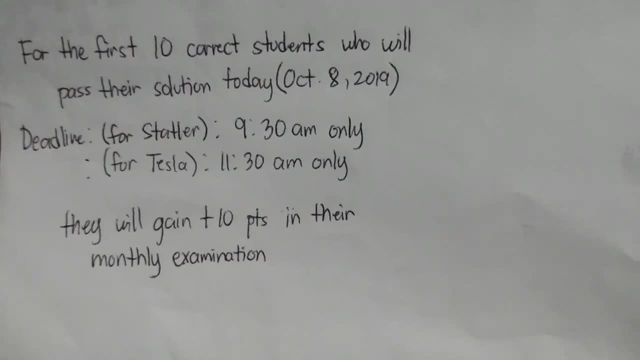 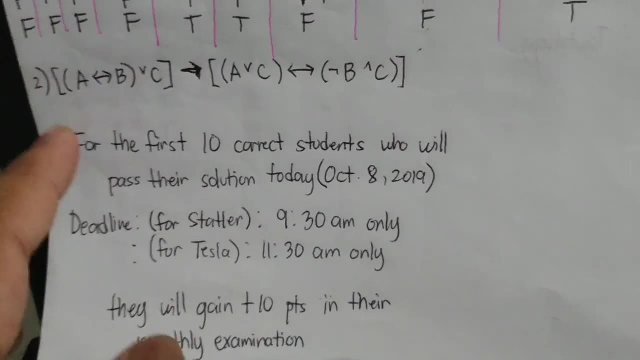 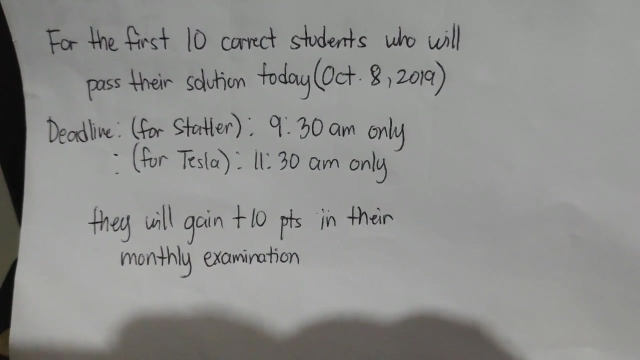 11, 30 am to pass it. so for those 10 students that you will, the first 10 students that you will get the correct answer for the proving for number two will have plus 10 points in their last monthly examination. again, this is for the monthly examination and i will only 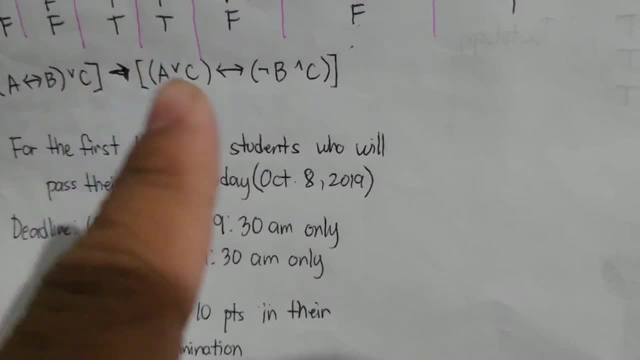 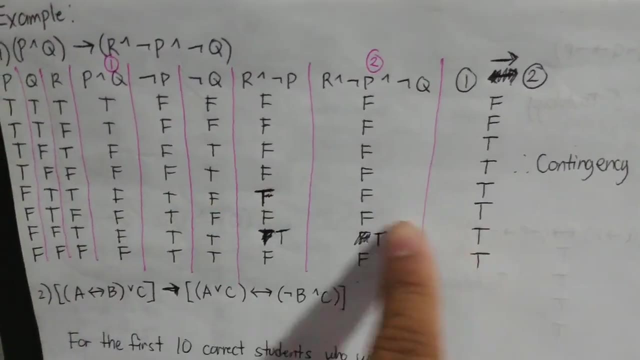 care for the first 10 students that you will get the correct answer for the proving for number two. so i will only give the full 10 points if we have all the correct solutions. so i need to see a replica of this one. so the solution must be like this and i will it check each, every statement. 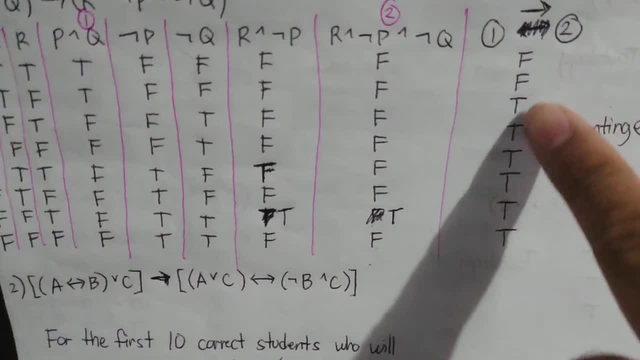 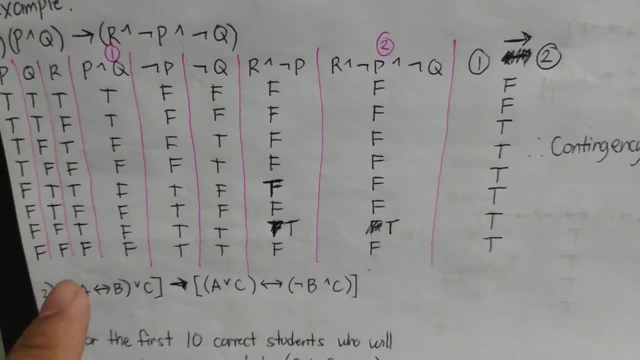 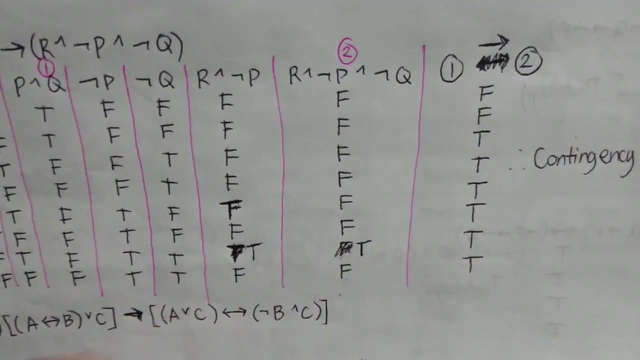 so i will not only consider the last part of the proving but also every column of your proving. again, you will be eligible to get the 10 points if all of the shoot values for your column are correct. so that will be the end of the discussion for lesson number three. for. 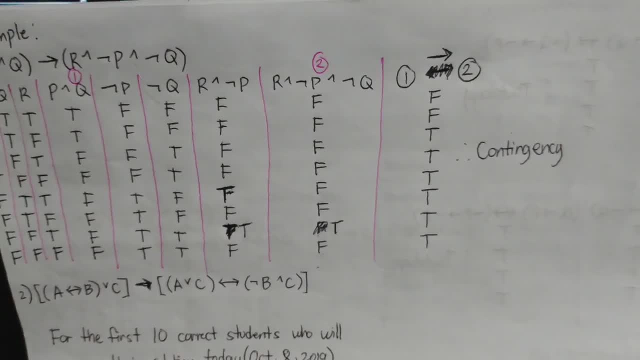 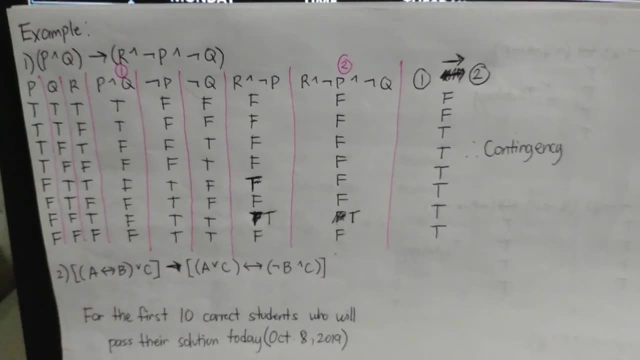 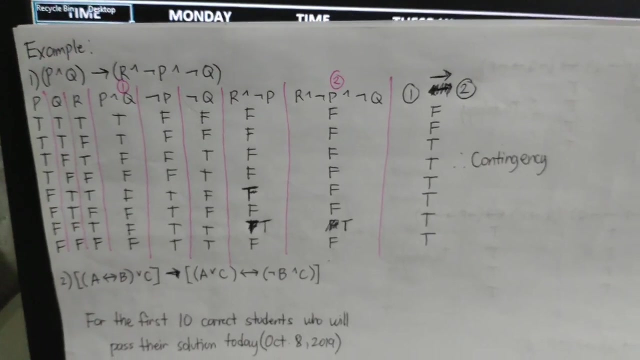 logic. so the subject teachers, or for the proctors that i will be substituting for me, will give you the activities that you need to do. so, again, i'm sorry for being absent at this time and i will promise to make it up for the succeeding 151. 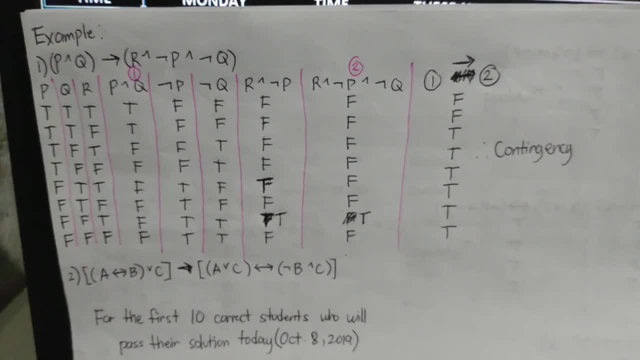 remain for the remaining days. Thank you.